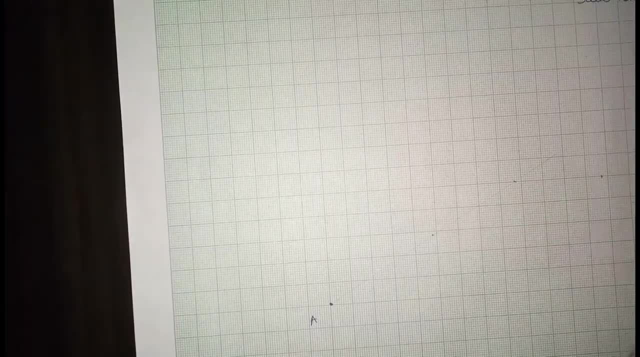 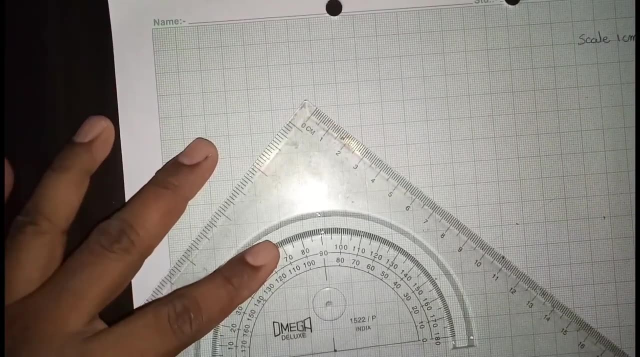 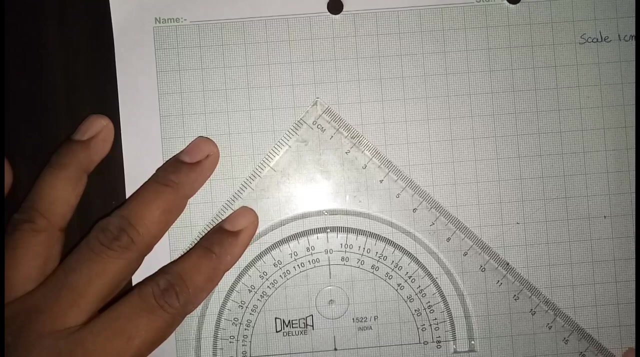 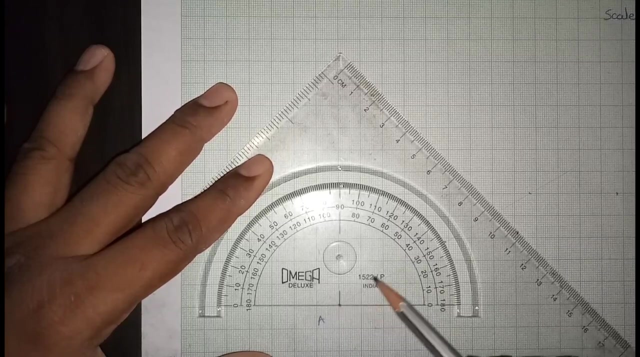 A point. Angle of slope is 30 degree. Angle of slope is 30 degree, So mark 30 degree with reference to this point. This is point A and this is 30 degree. This is the 30 degree point. This is the baseline. 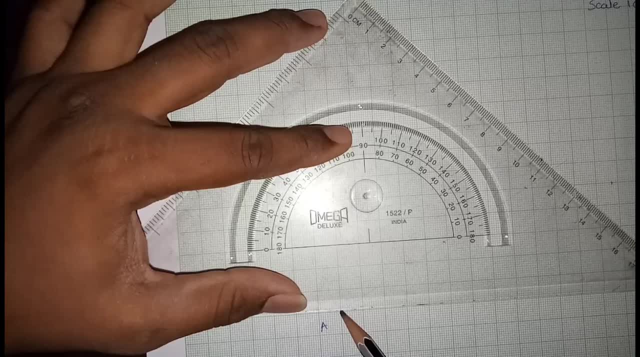 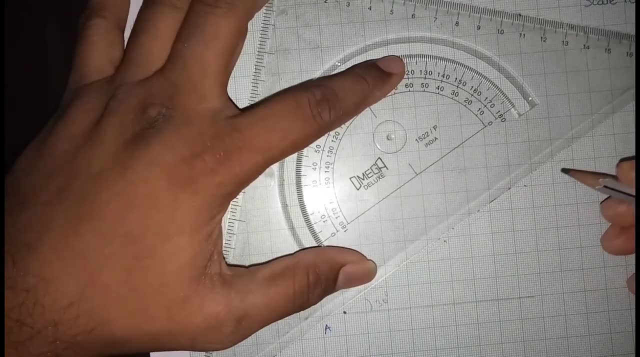 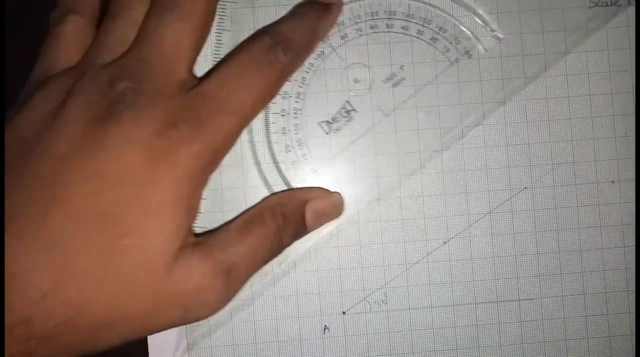 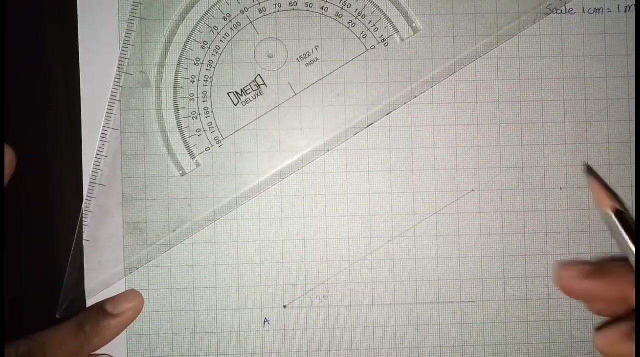 Angle of slope is 30 degree, So mark 30 degree. with reference to this point, This is the. With reference to this, this is 30 degree. mark 30 degree. Now, depth of cut is 5 meter, so height of slope is 5 meter. our scale is 1 cm, is equal. 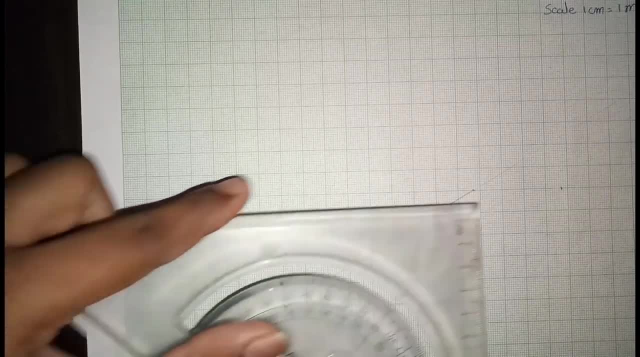 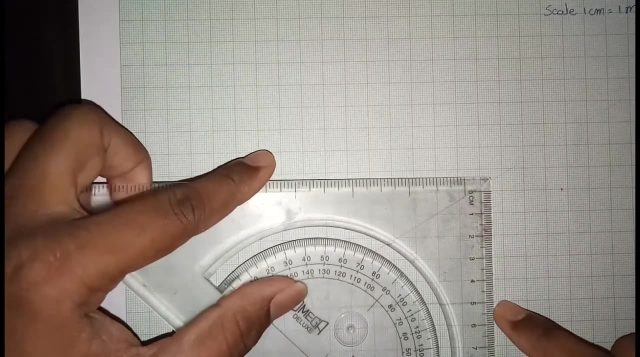 to 1 meter. so 5 cm is equal to 5 meter. so this is your base line. select 5 meter from this where it is intersecting. so this is 5 and this is 0, so it is intersecting somewhere. 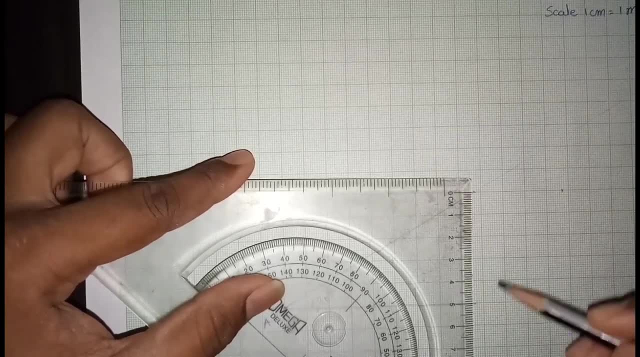 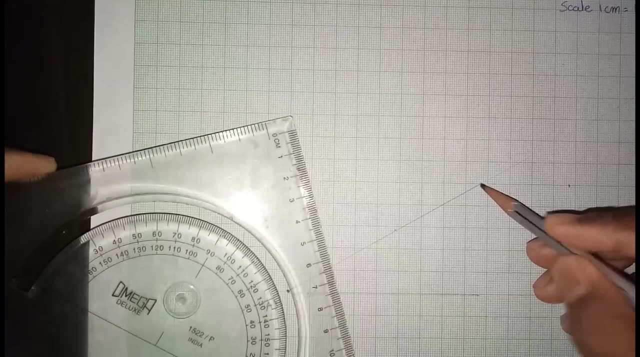 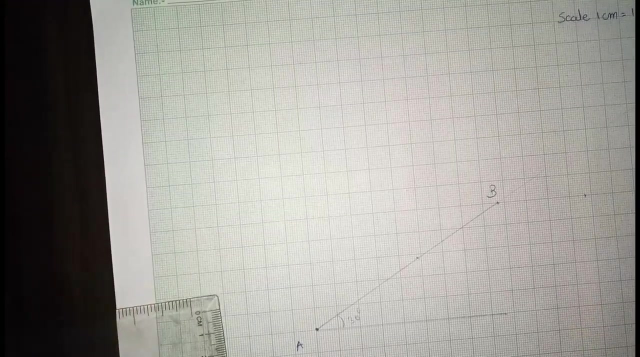 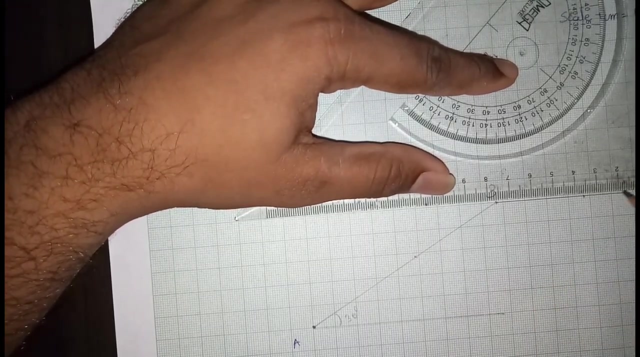 here. so this is your height. from here to here is 5 meter. so select 5 meter point on the inclination. so this is your end point. this is height of embankment. This is point B and draw horizontal line. so this is the embankment. this is the inclination. 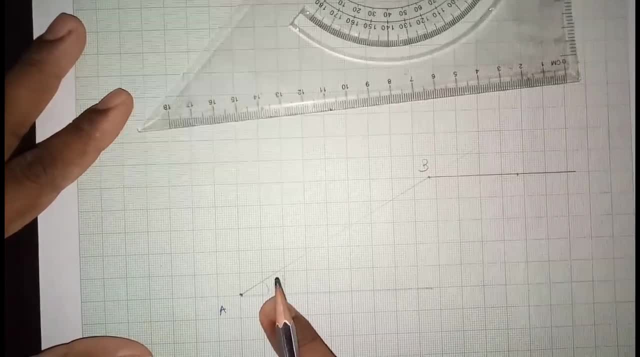 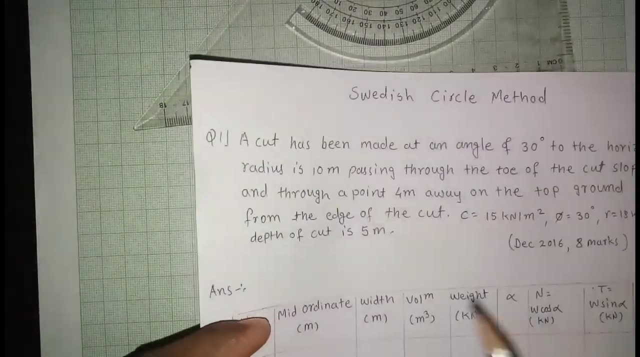 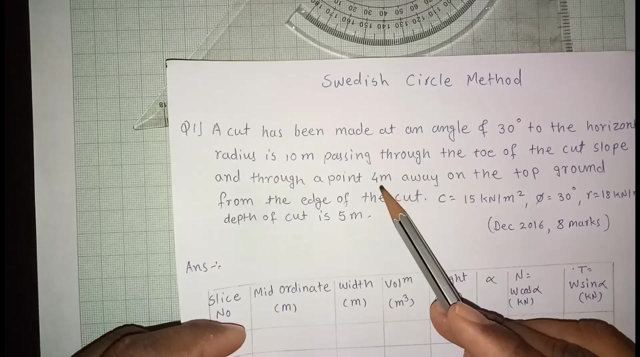 slope 30 degree and this is the base of the embankment. ok, Now this point is cutting at top point is cutting at 0., 4 meter away on the top ground. so this is the 4 meter distance. so 1 cm is equal to. 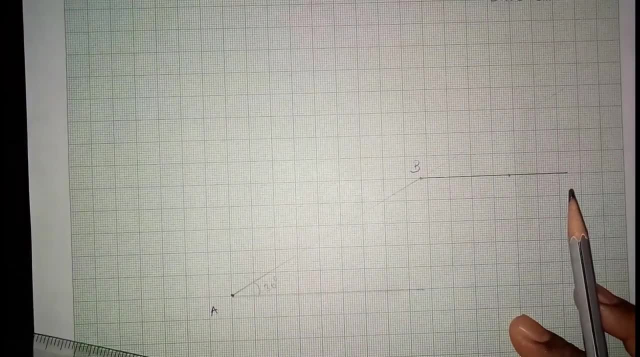 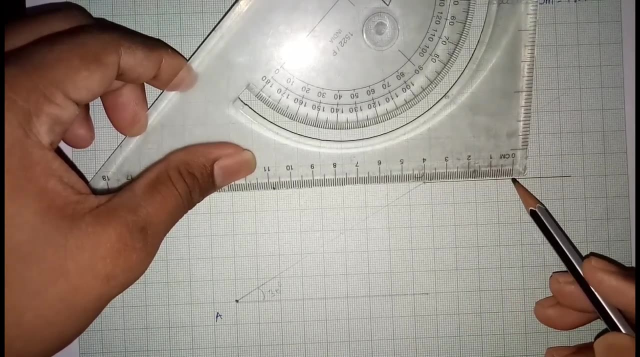 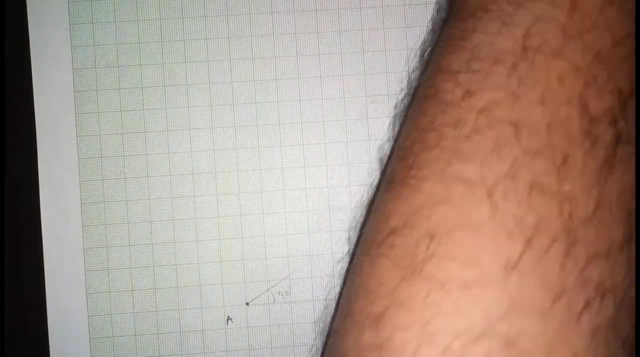 1 meter. so 4 cm is equal to 4 meter. so this is 4,, this is 0, so this is the end point. so A, B, C Radius is given to us. radius is 10 meter. 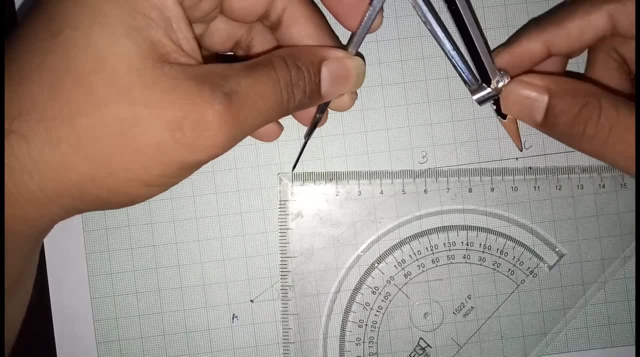 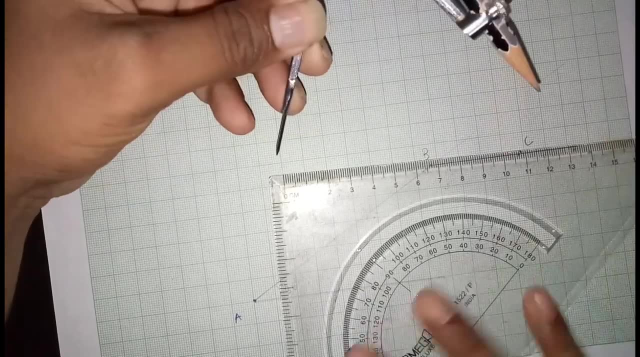 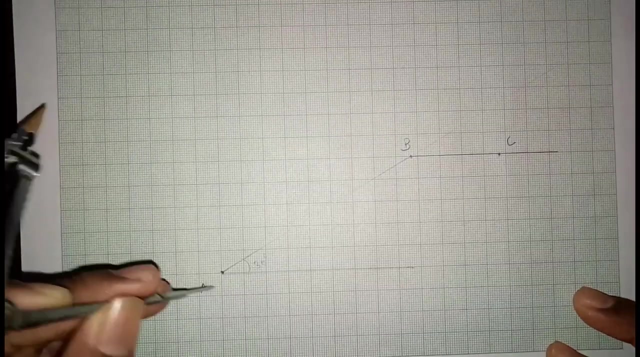 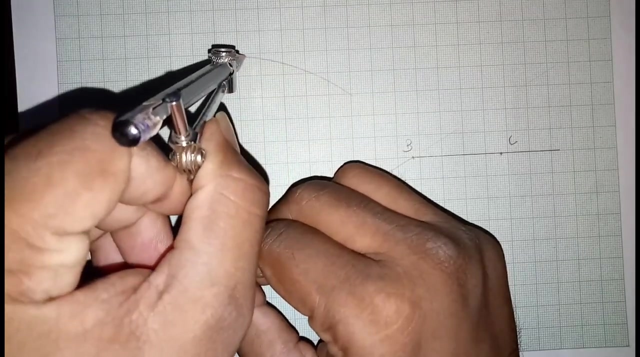 so this is 0, and this is 10,. so this distance is: take 10 meter once. take a 10 meter distance in your compass. keep one point at A stationary point and draw the arc. keep point on C. 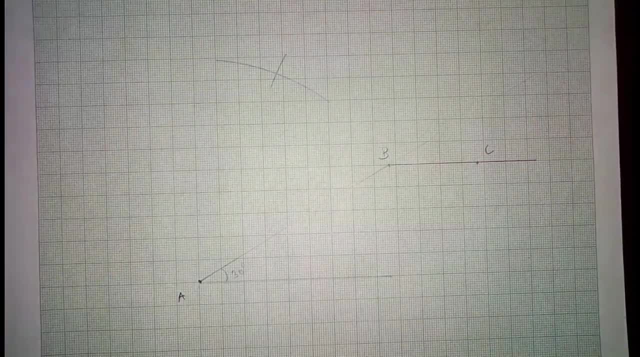 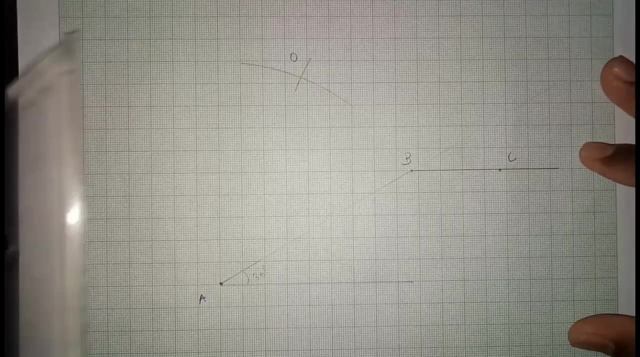 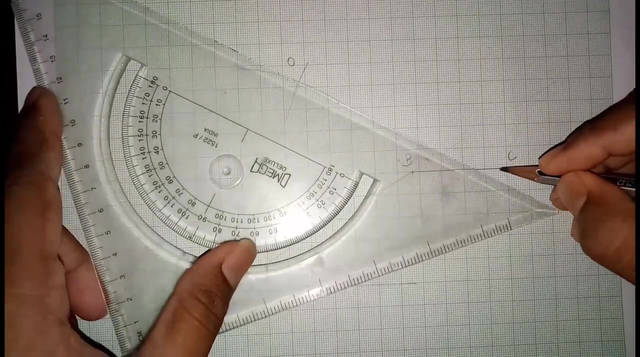 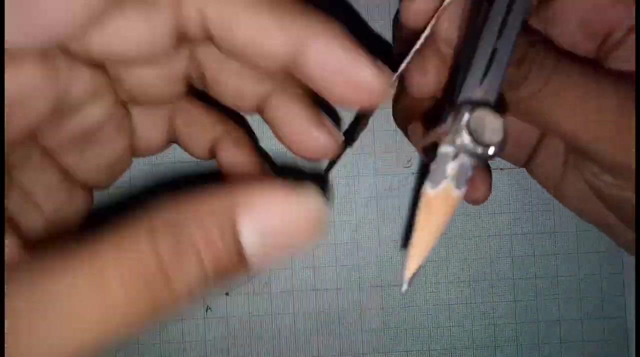 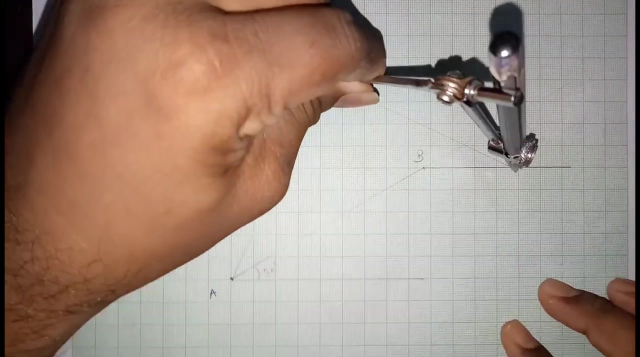 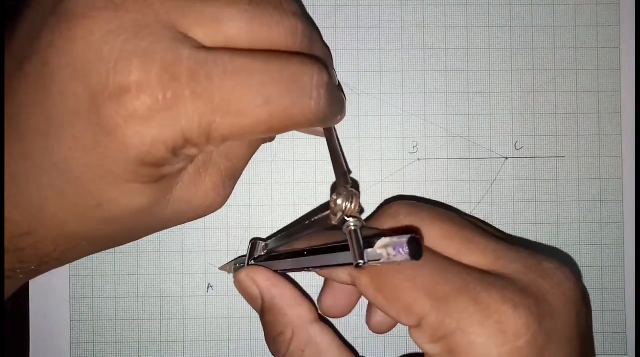 again draw the arc. this is point O. join the line O, A and O C, O, A and O C. so draw the failure surface, the keeping point on O at C and at A. join A and C by semi-circle. so this is your failure surface. this is a. 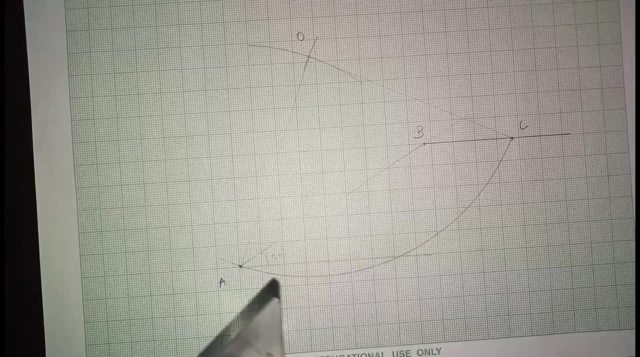 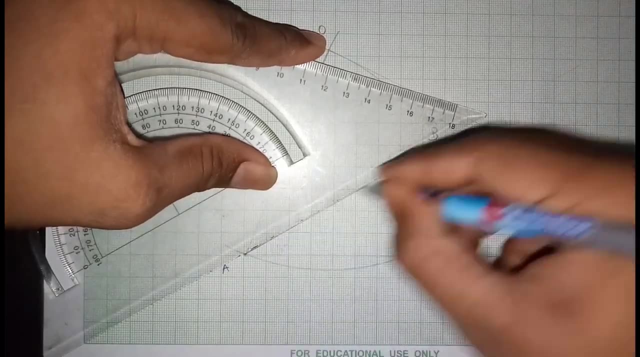 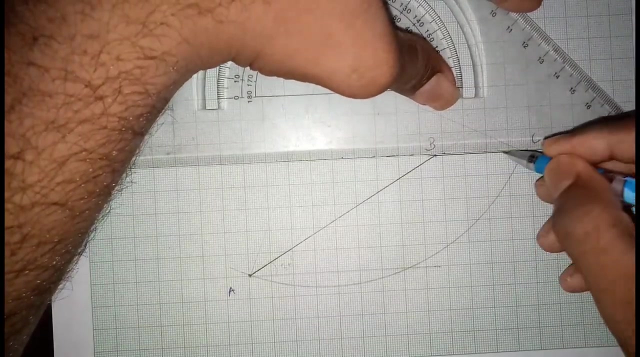 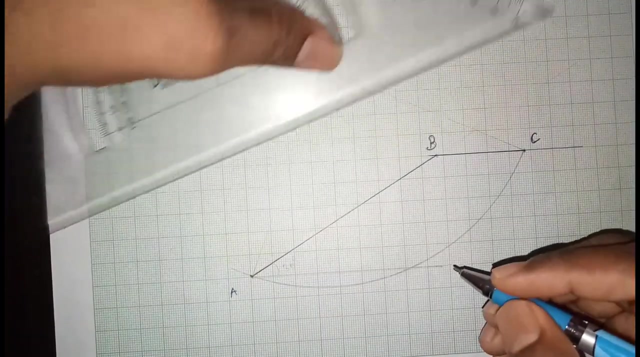 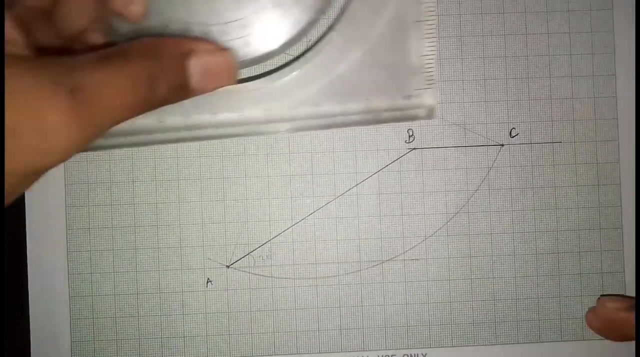 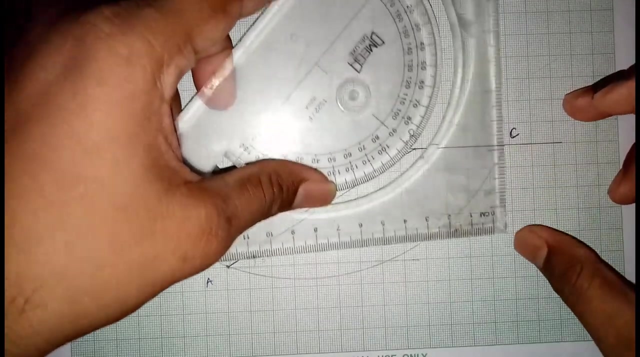 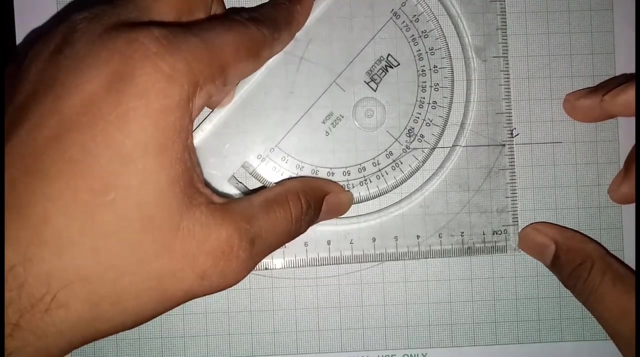 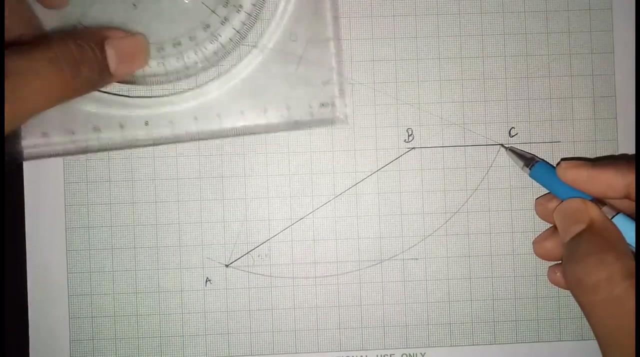 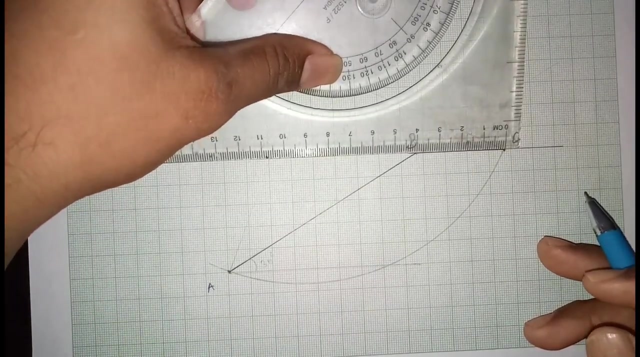 slice, failure slice. Ok, this is your slope now. total length of this failure surface is 3,. that means from here to here is 12.5 meter. The total length from C to A. total length from C to A is: 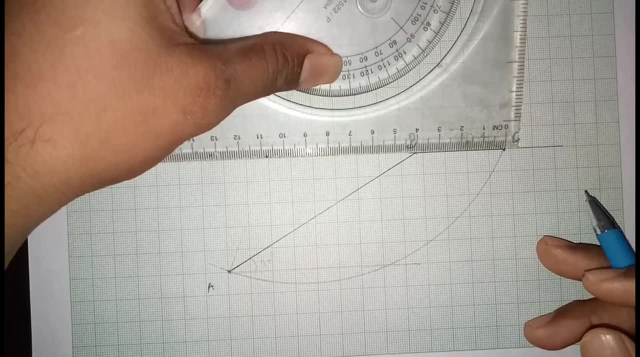 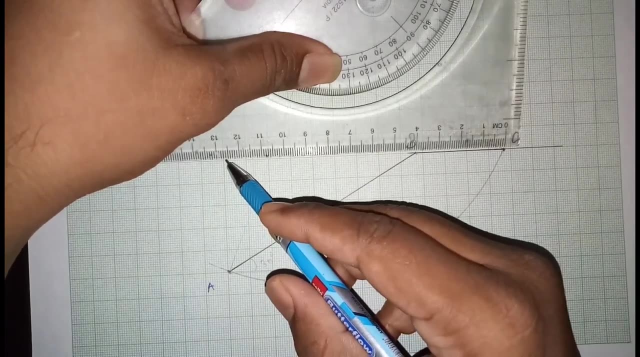 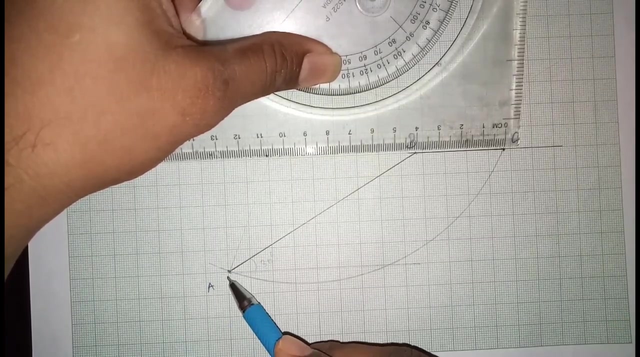 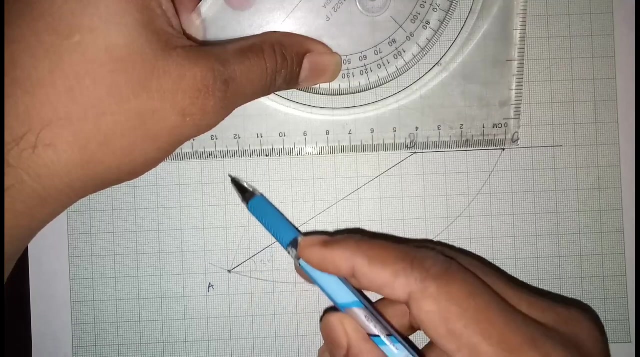 12.5 meter. 12.7, ok, 12.7 meter. The total length from 12.5 meter- 12.7 meter a to c or c to a, is 12.7 meter. okay, this is a, so this is 12.7 meter from. 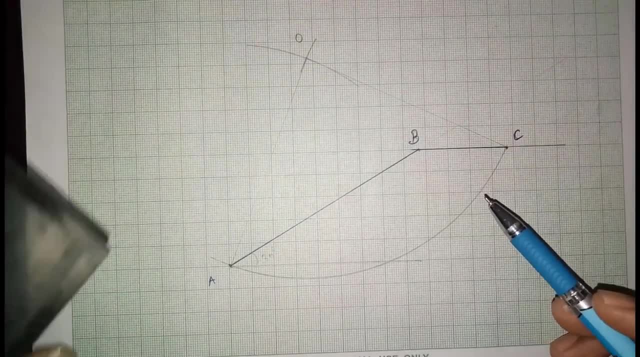 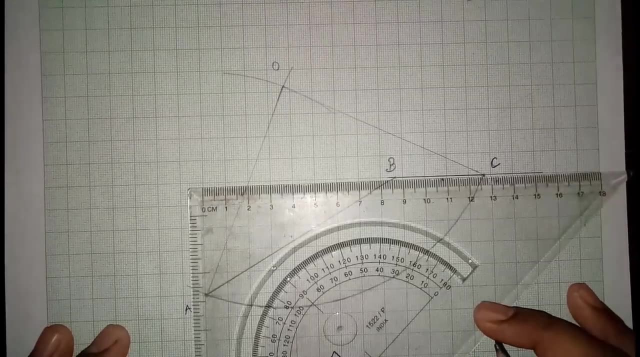 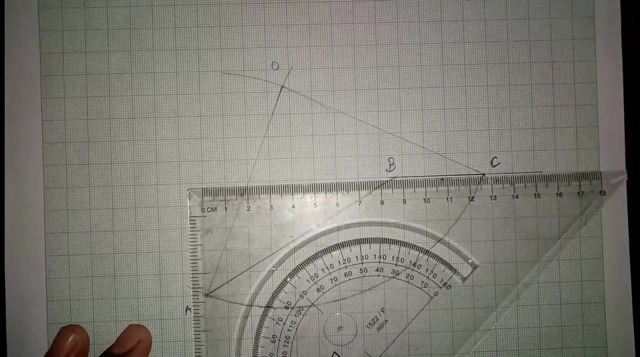 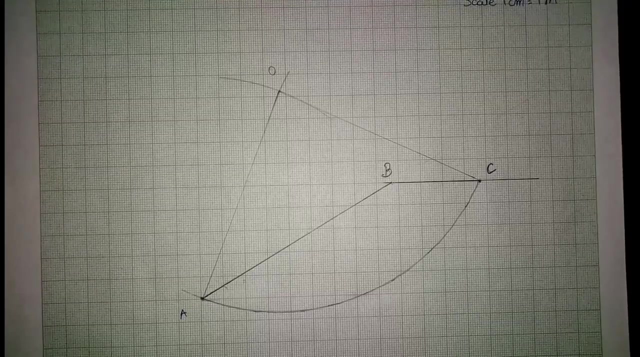 c to a. now we have to subdivide it. we have to subdivide the whole distance. total distance from a to c is 12.7 centimeter. so here we have to make a slices of this sections. So we can make 6, ,7,8 slices, depending upon the requirement or as some number of 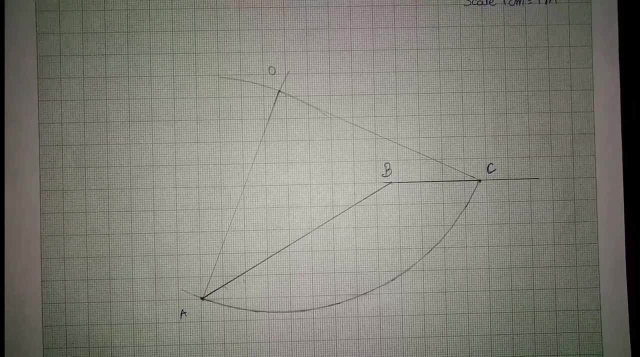 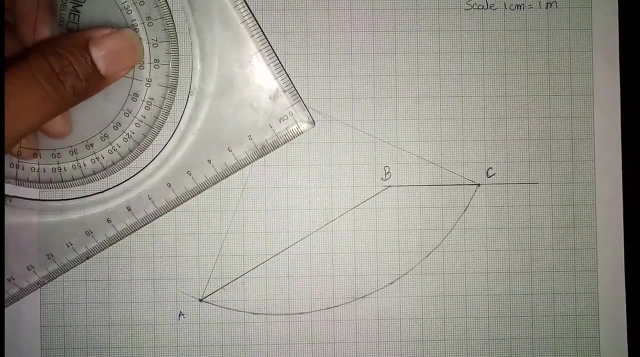 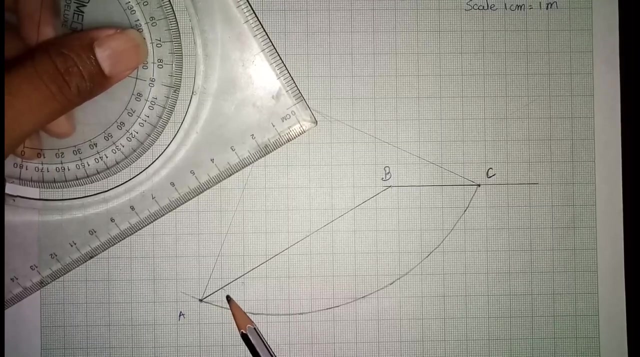 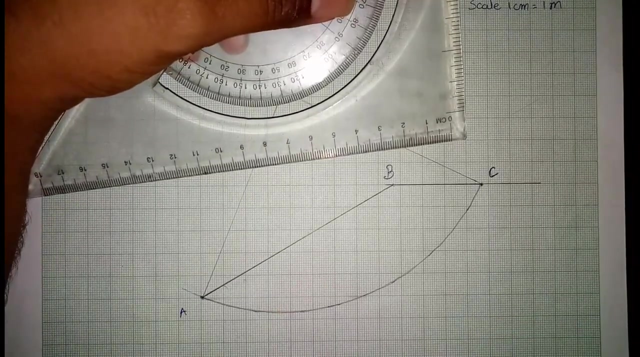 slices increases, result will be accurate. so approximate: make 5 to 6 slices. so we will make 6 to 7 slices. so total distance is 12.7. so 2 meter per slice. We will make 2.7 meters per slice, so number of slices will be seven. two meter till 12 meter. two meter per slice. 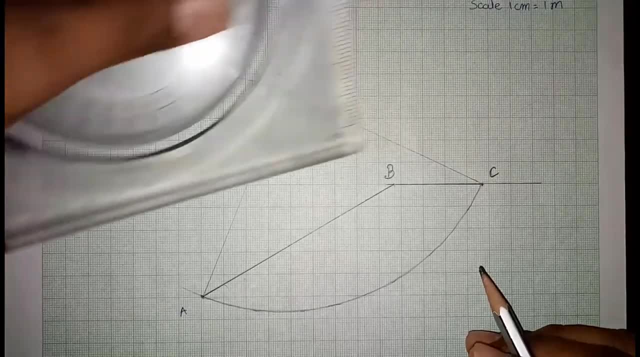 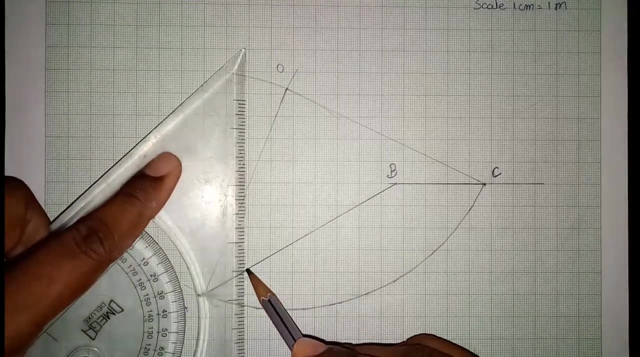 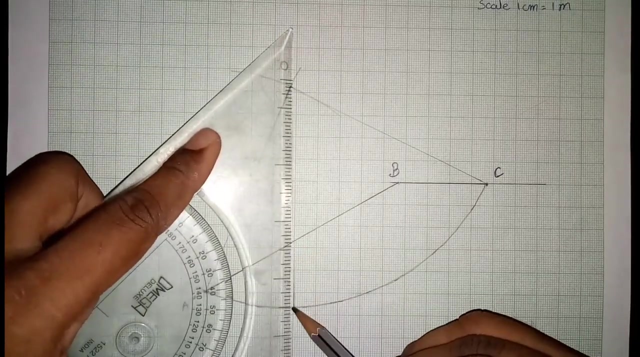 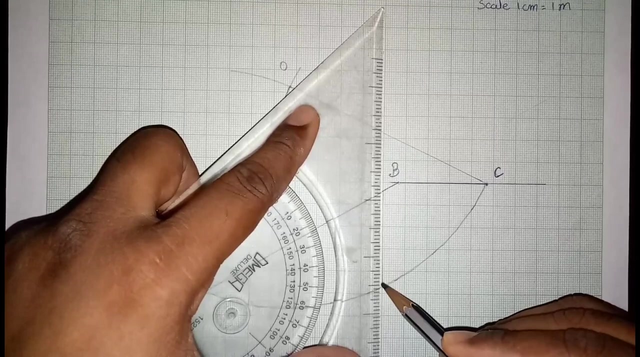 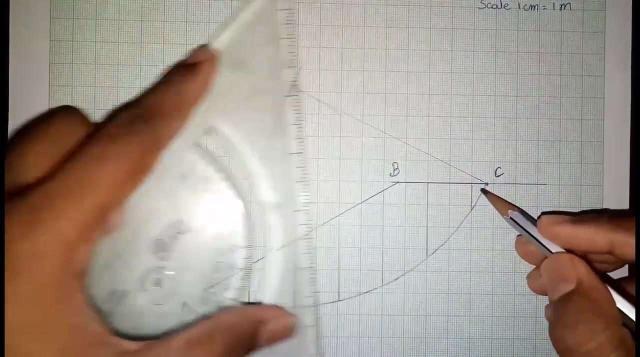 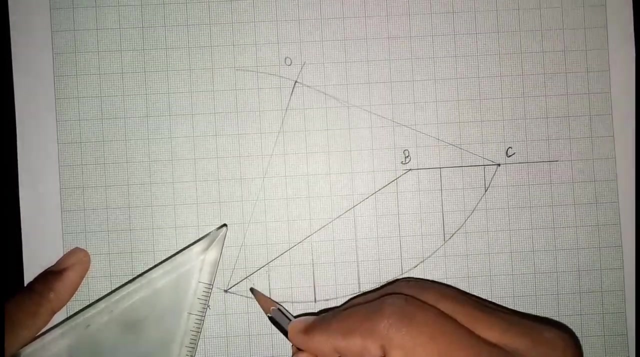 is so this is zero. one meter, two meter. so we will make one slice here, draw a straight line and join the top and bottom portion. one meter, two meter. again. second slice, third, fourth, fifth and six, and this remaining potion is for 7th number of slice. ok, this is 1. 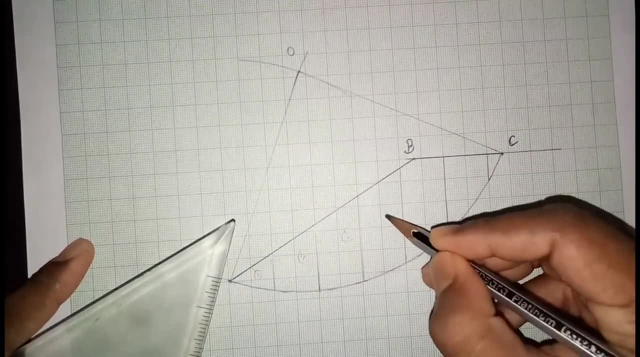 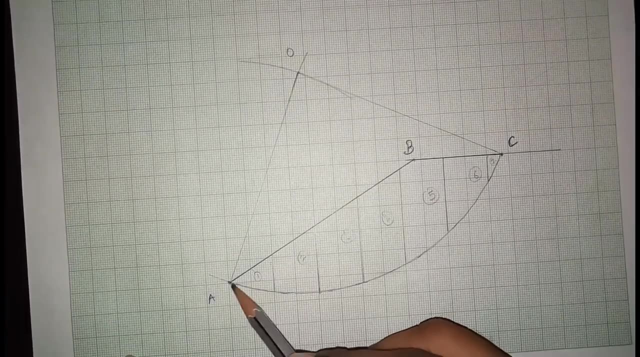 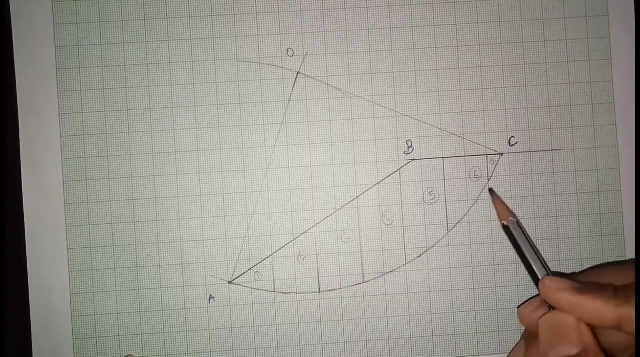 2, 3, fourth, fifth, 6 and last one is 7, so this first to 6 number of slices are having width 2 meter. each slice having width 2 meter. that means up to here, from here to here, is 12 meter and remaining 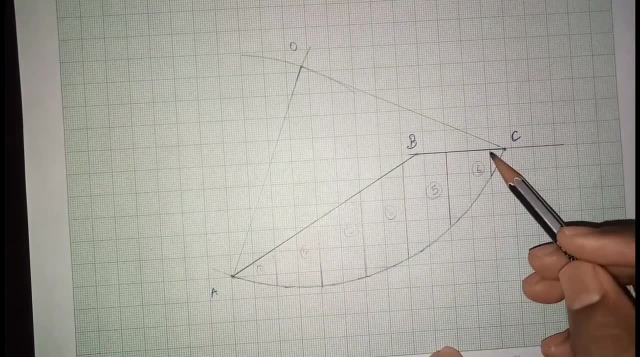 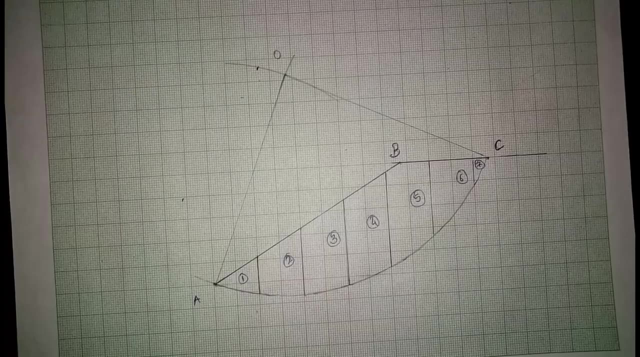 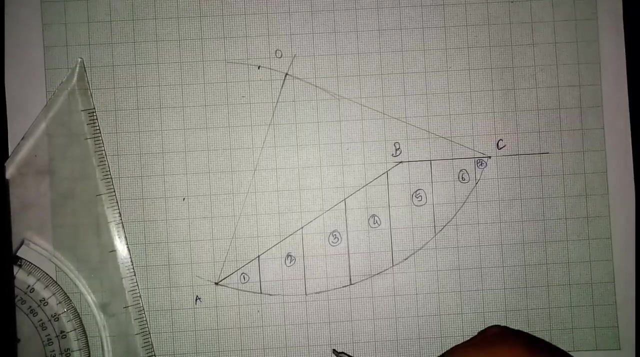 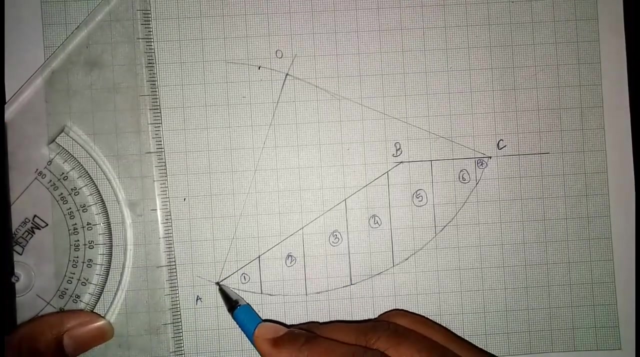 0.7 meter 7 slice having with 7 meter. so after doing slices, draw the mid-ordinate, mid-ordinate in between. mid-ordinate is the center of the slice. so this wise start from here in here. so Sag полож ginger mov 44 norm. 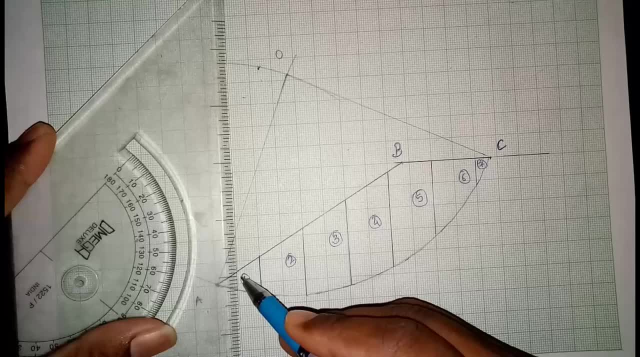 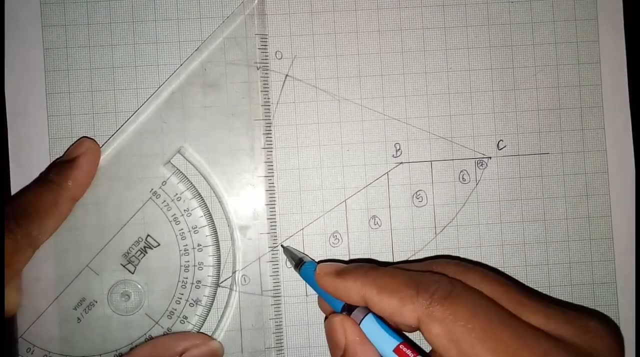 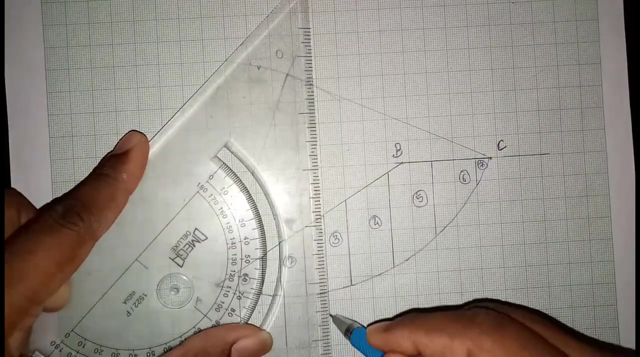 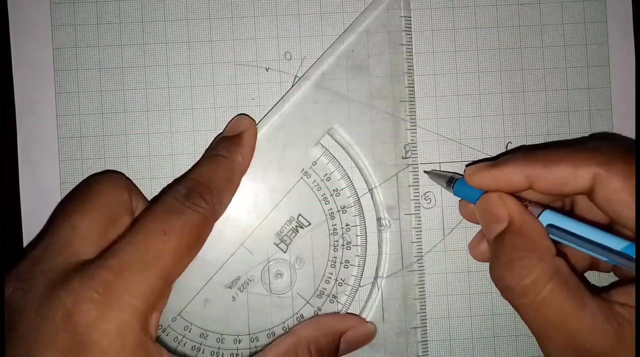 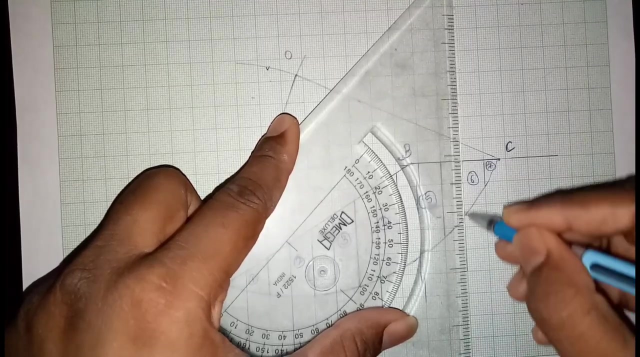 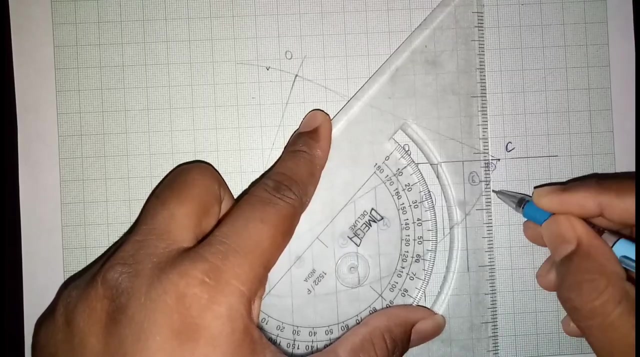 economic index. the center of this lies 백신和水平, and extend Record point to between: mid ordinate is the center of the slide, so small cut has 3 Best flash value: the mid ordinate line. these are the mid ordinates. mid ordinate has been drawn. 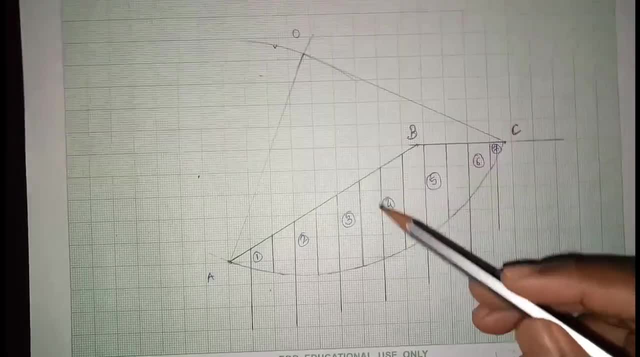 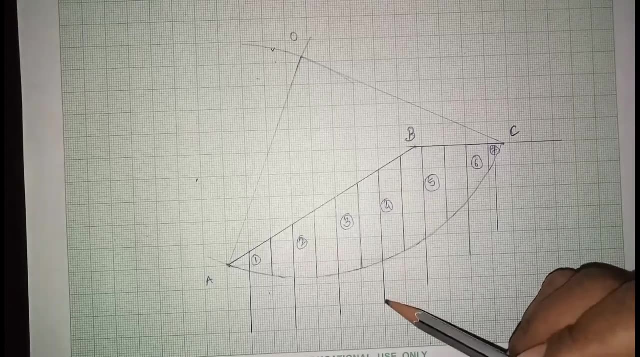 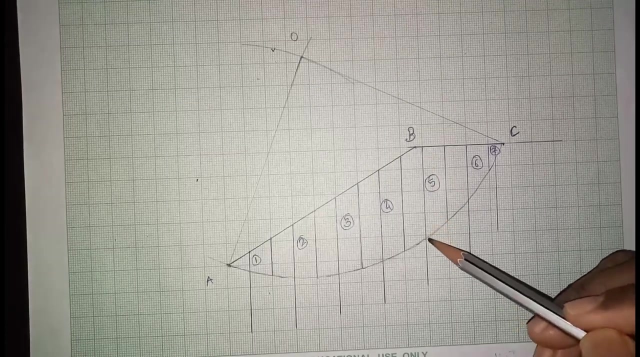 these are the mid ordinates. this is the width of the slash. length of the fourth number. slash length of the mid ordinate. length of mid ordinate from here to here. length of mid ordinate for before, below, below, below, below. Slice number 4: from here to here. 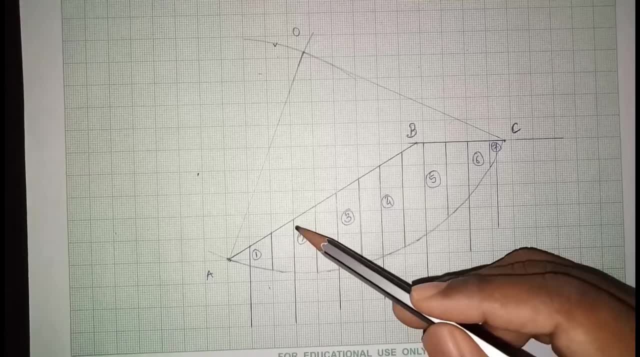 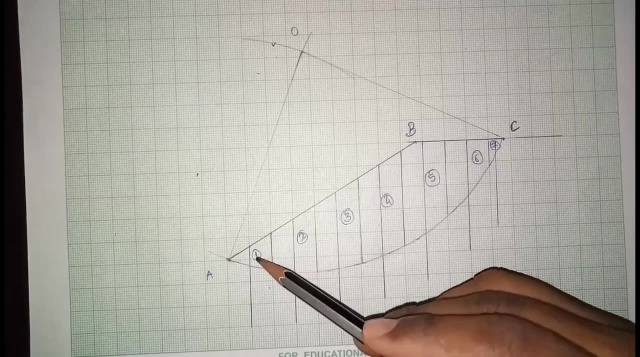 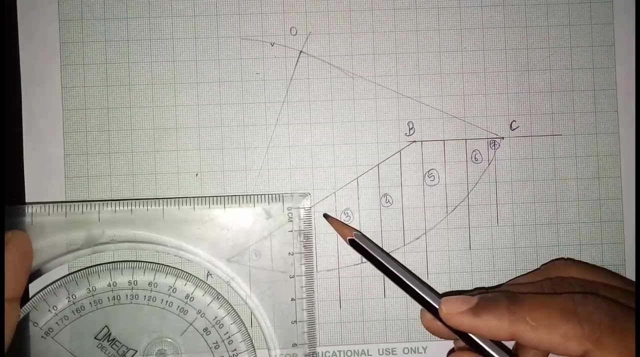 Length of mid ordinate for slice number 3 is from here to here. Length of mid ordinate for slice number 2 is from here to here. So we have to measure length for all the slices. We have to measure the length with the help of scale for all the sizes. 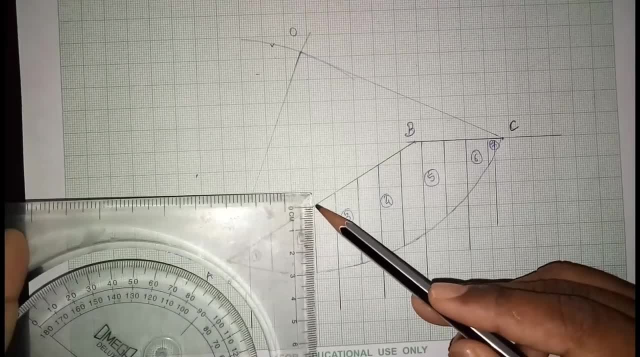 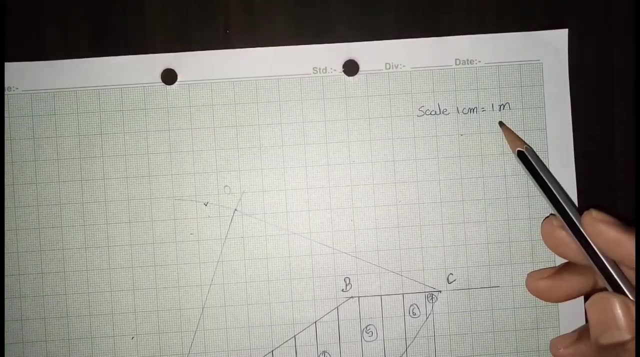 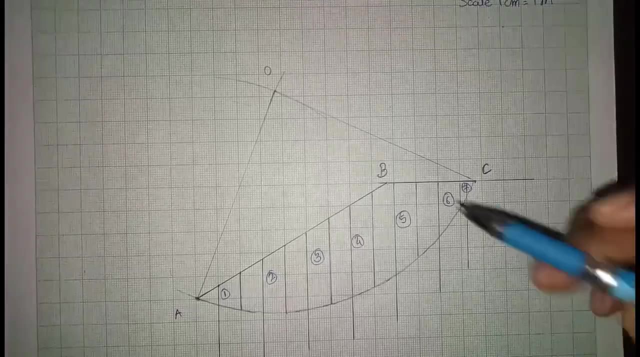 This is slice number 2 from here to here. So length of mid ordinate for slice number 2 is 3 cm. That means 3 meter because our scale is 1 cm is equal to 1 meter. Now draw the angle with respect to O. 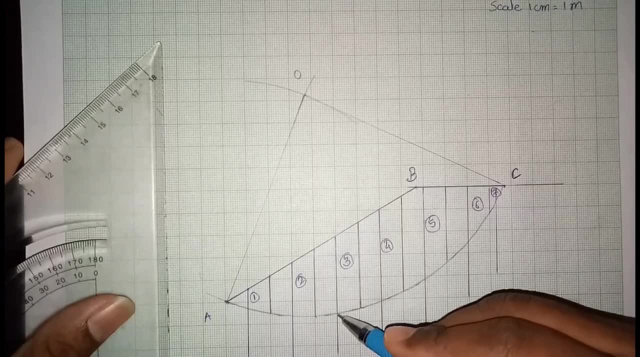 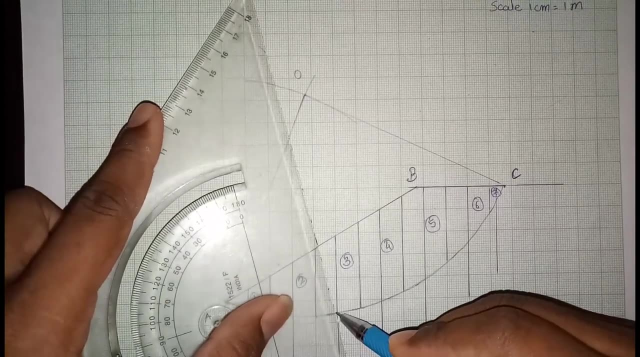 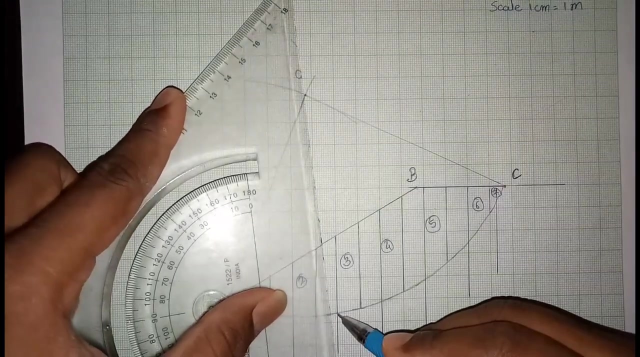 Now, here we can see that if we consider slice number 3.. Now, this is the mid ordinate center And, with reference to this point, and with reference to this point, This is point O And this is mid ordinate of slice number 3.. 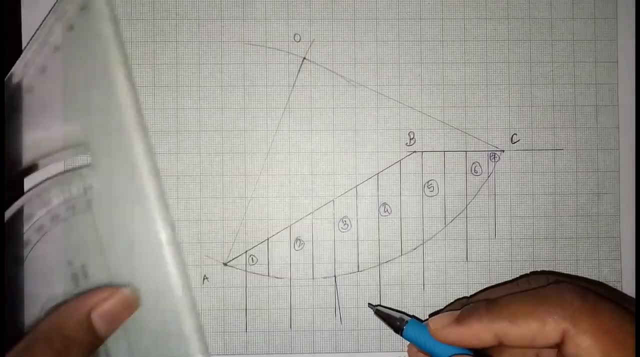 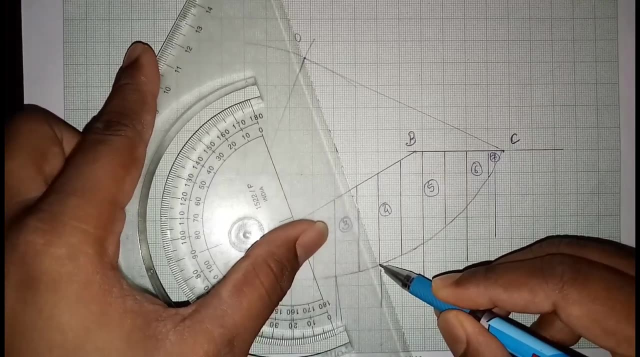 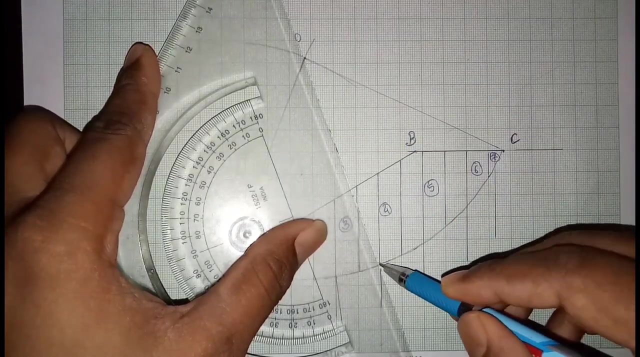 Draw the angle. So this is the angle. Now for slice number 4.. Again, same. Keep one point here. and with reference to point O, This is O point. This is the mid ordinate of slice number 4.. Draw the angle. 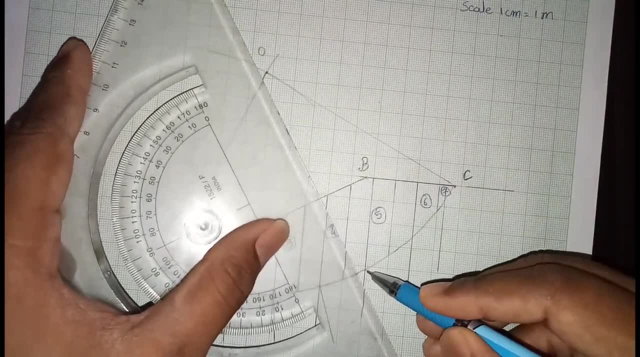 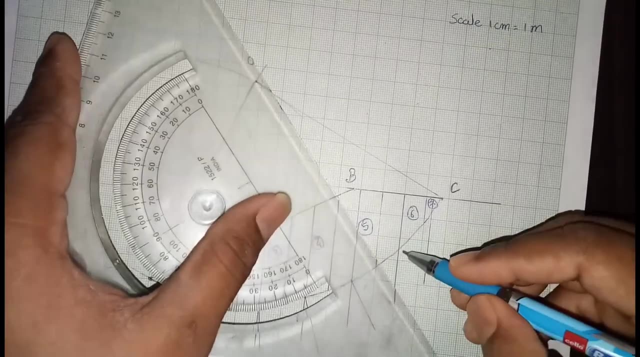 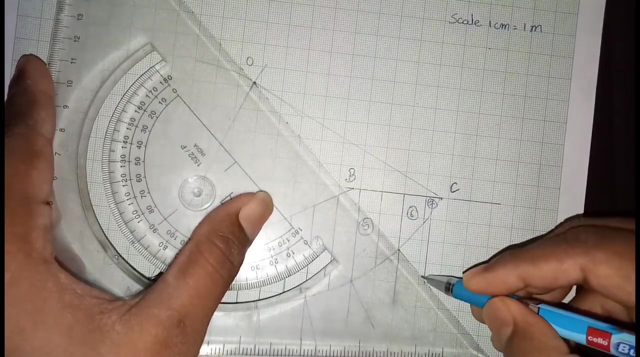 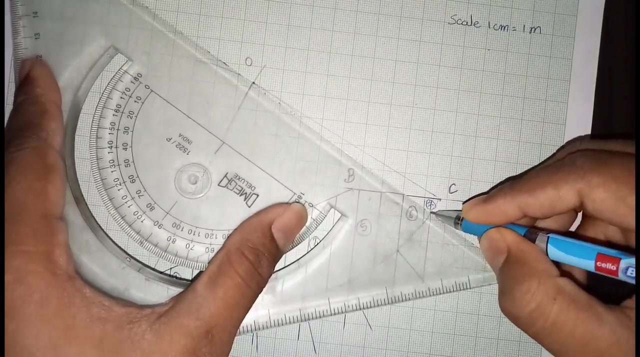 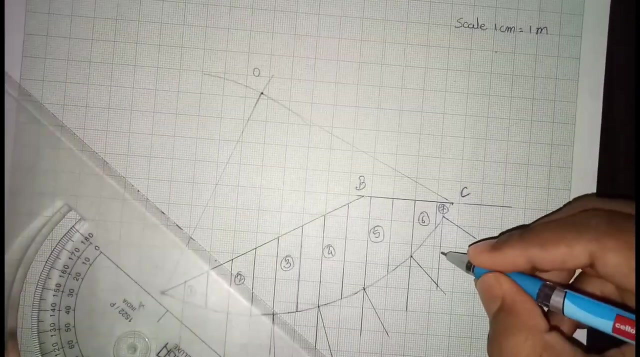 Likewise we have to do for all the slices. Keep it At the center. With reference to O, Draw the angle Again, same. After that we have to measure that angles also. This is for slice number 7.. So this downward, vertical downward indicates: 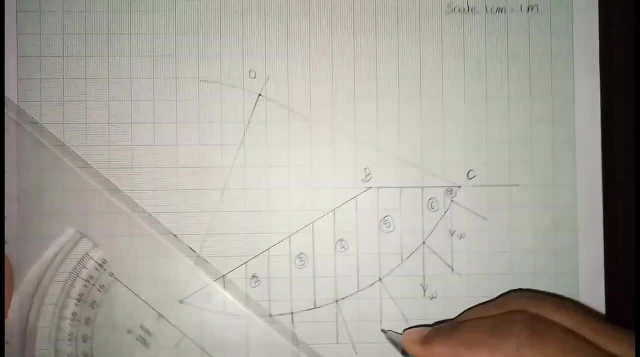 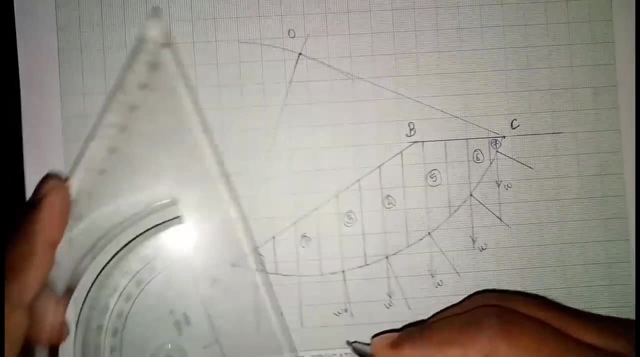 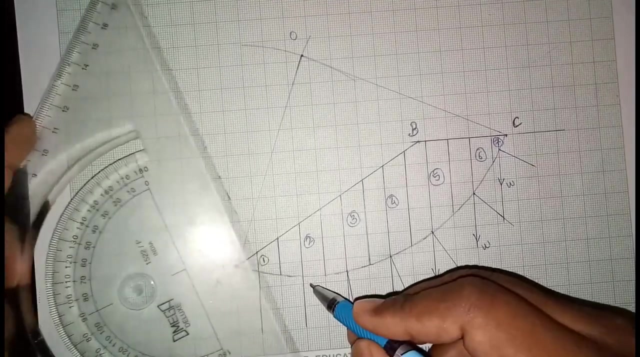 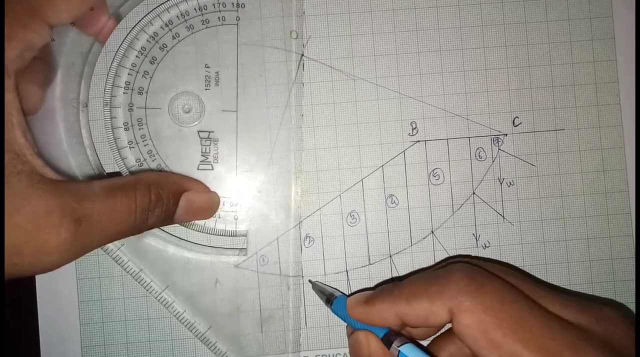 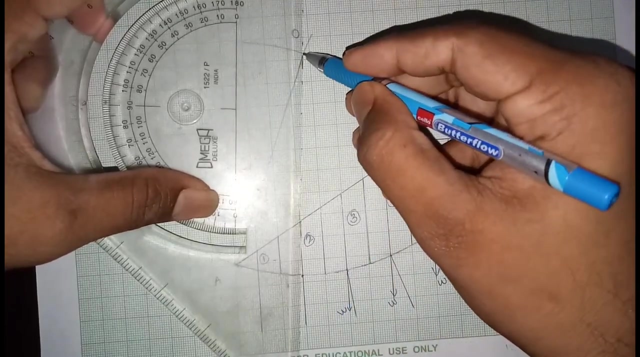 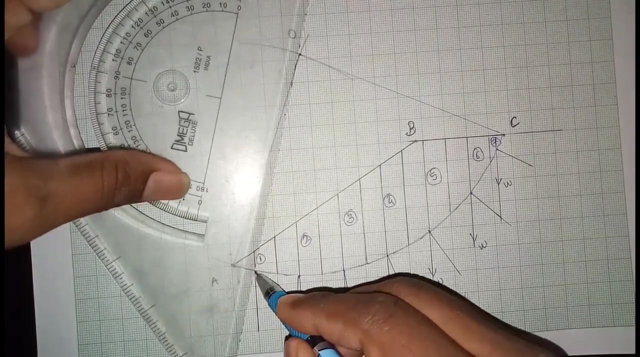 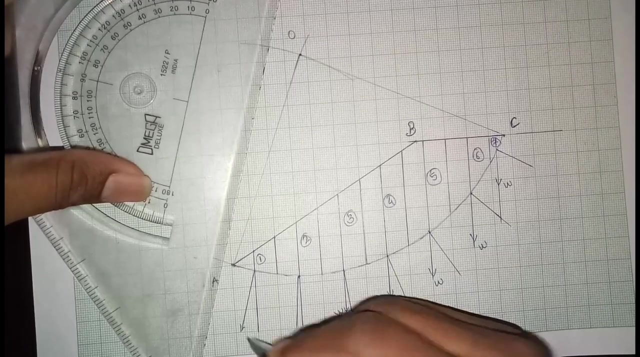 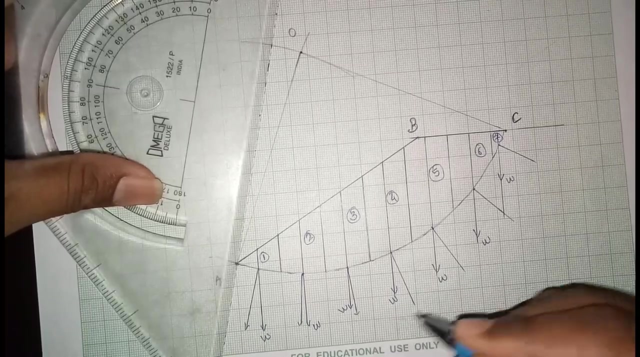 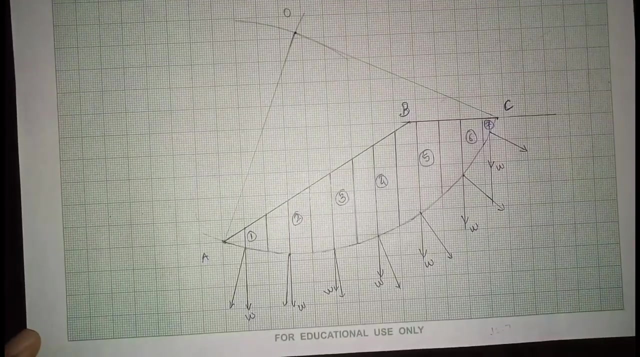 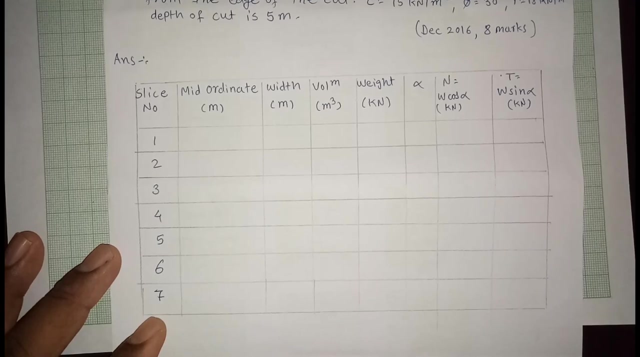 W- Weight of the slice. W. This vertical downward arrow indicates W, That means weight of the slice. Ok, here now the angle changes from right hand to left hand. Okay, After drawing this all angles, then we have to measure the all the angles. 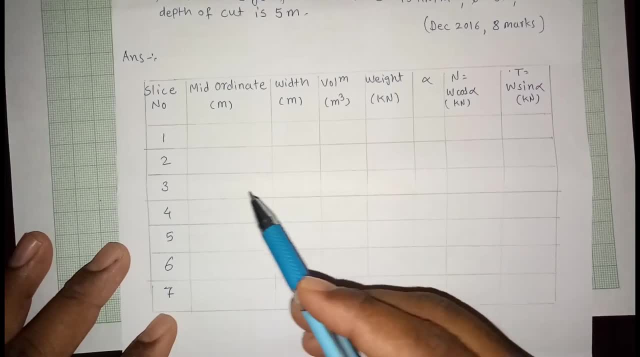 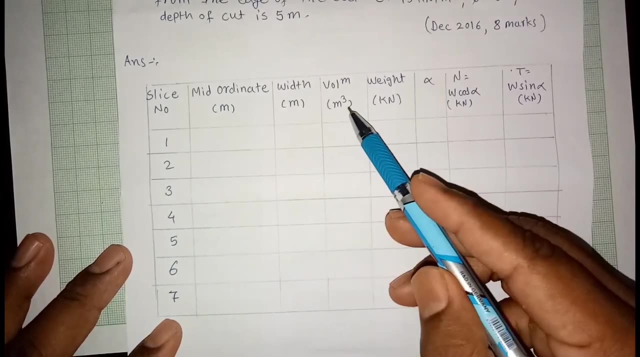 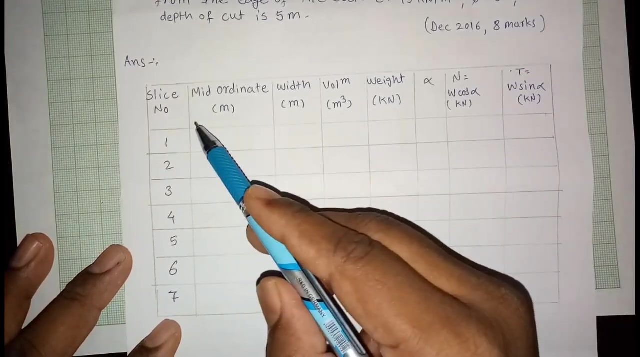 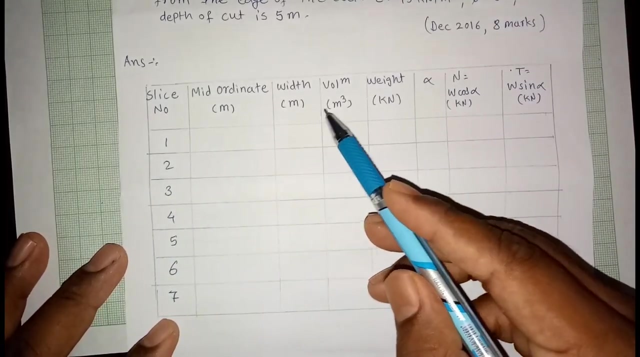 After drawing graph, make a table having content: slice number: mid ordinate. length of mid ordinate in meter. width of mid ordinate in meter. volume of mid ordinate in meter. cube. weight of sorry slice: number- Mid ordinate in meter. width of slice in meter. volume of slice in meter cube. weight of slice. 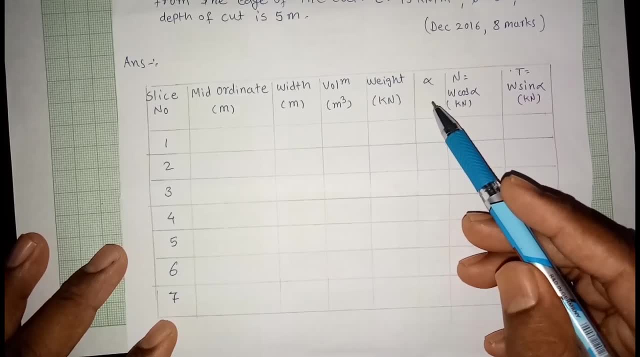 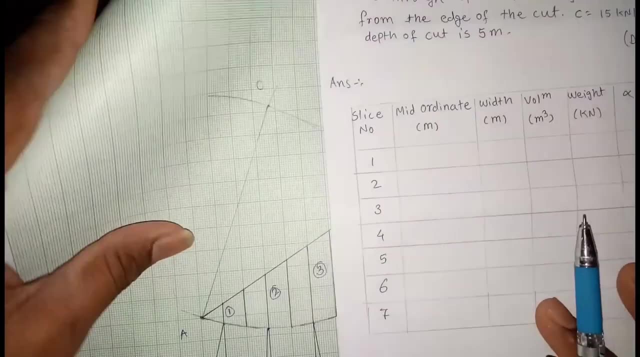 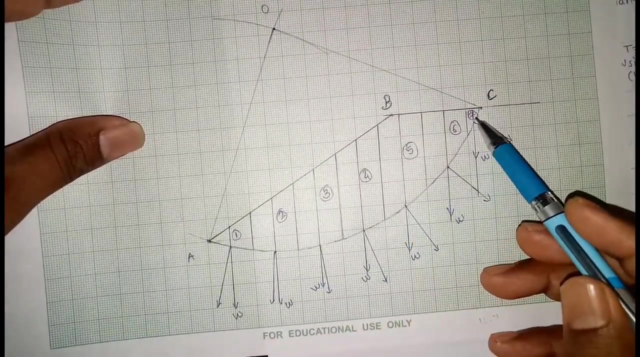 in kilo Newton. This is the alpha angle, normal and tangent. Okay, So we have a seven slices here. We can see that number of slices are seven: one, two, three, four, five, six and seven. So number of slices seven. 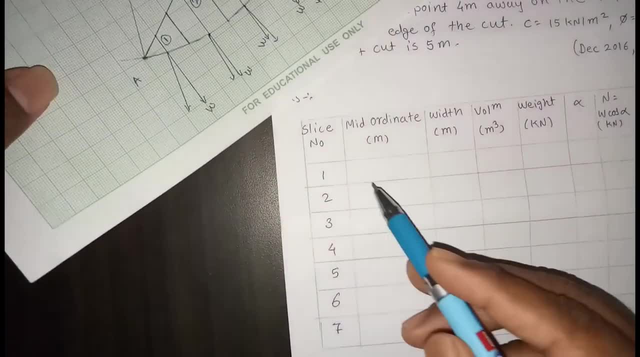 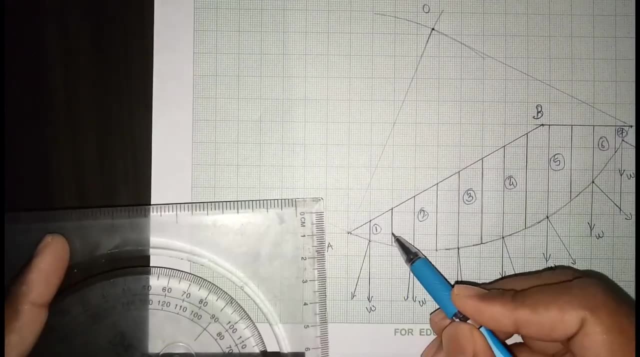 Now we have to Calculate the mid ordinate length For slice number one. the mid ordinate length is. we have to measure This is the middle. This is the total width of the mid ordinate- sorry, total width of the slice number one. 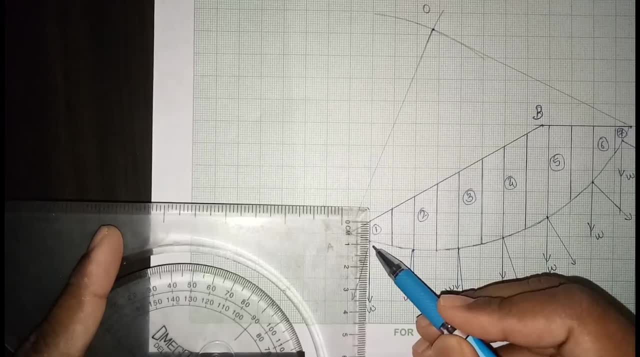 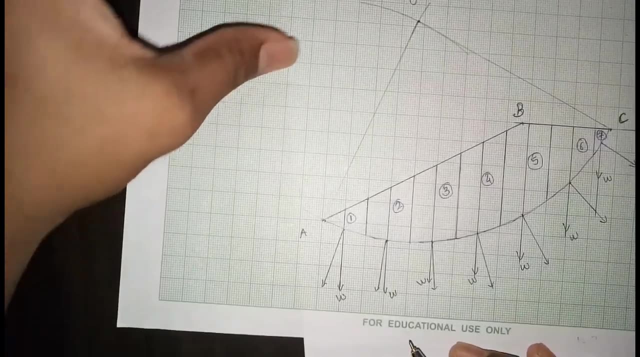 This is the mid ordinate, and length of mid ordinate is for slice number one, is eight centimeter. That means 0.8 meter, because our scale is one centimeter is equal to one meter. So for slice number one, the length, 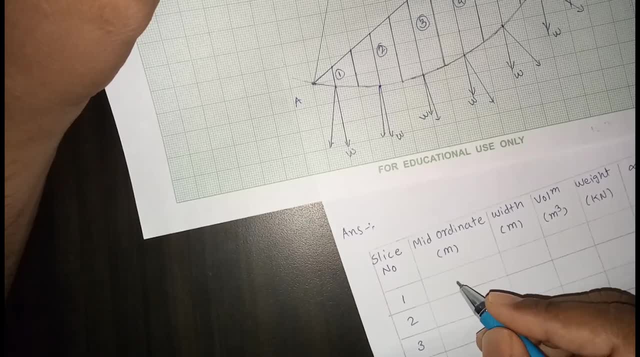 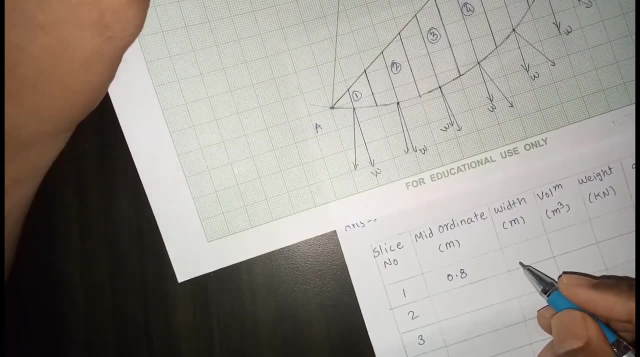 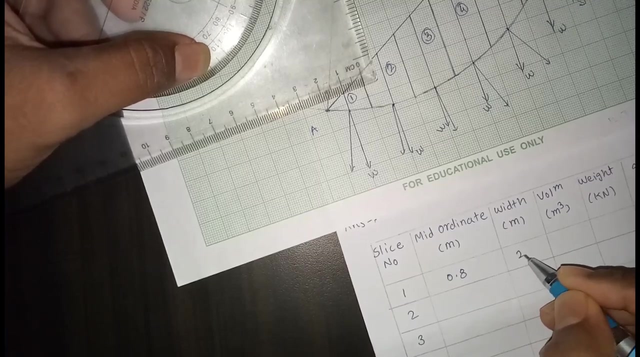 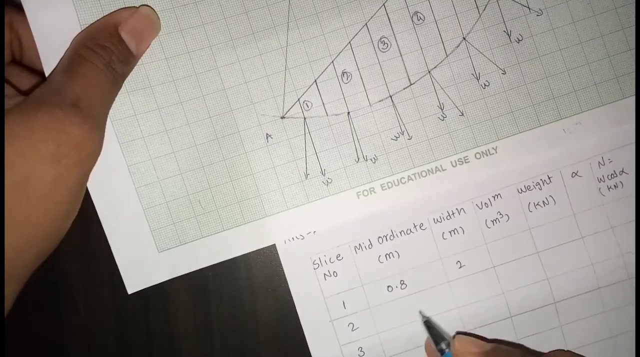 Length of the length of the mid ordinate is 0.8 meter And width of the mirror slice number one is two meter. one to two meter. Now for slice number two. Width of slice number two is again same. Width of slice number two is again same. 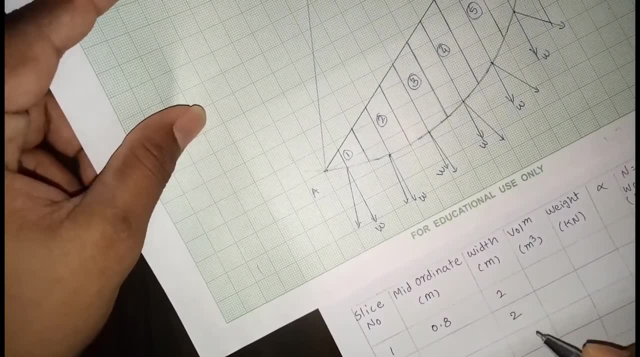 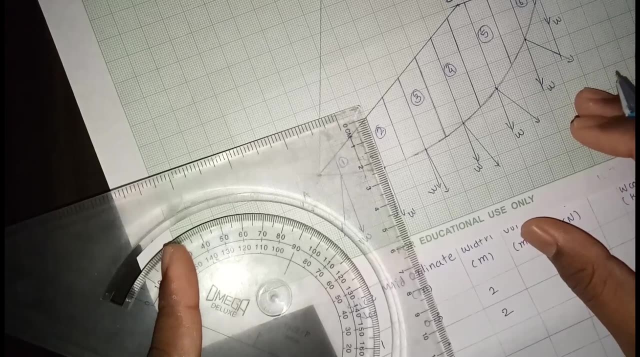 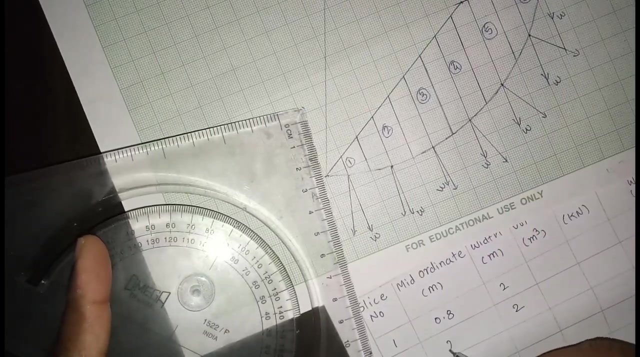 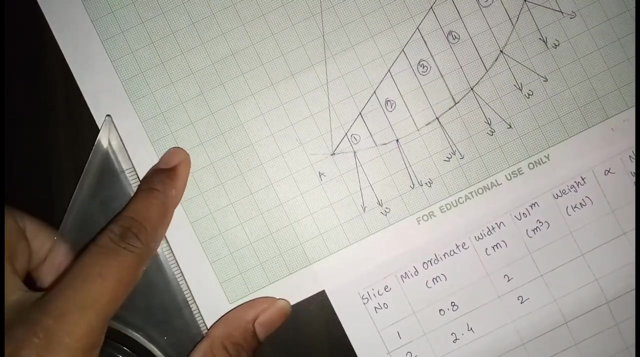 Width of slice number two is two meter and the length of the mirror ordinate for slice number two is 2.4 meter, from here to here: 2.4 meter. Now consider the slice number three. slice number three and length of the mirror ordinate. 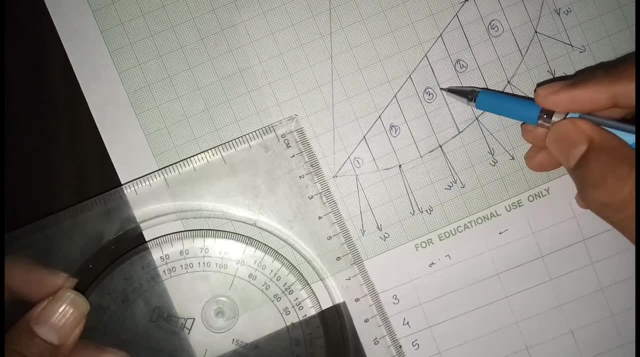 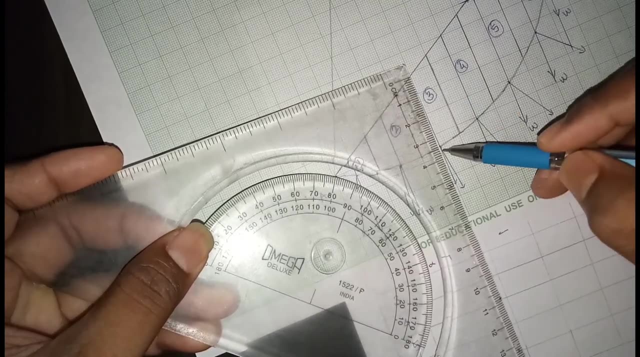 for slice number three is: this is slice number three from here to here, And length of the mirror. ordinate for slice number three is: this is zero, 3.5.. Length of mirror. ordinate of slice number three is 3.5 meter. 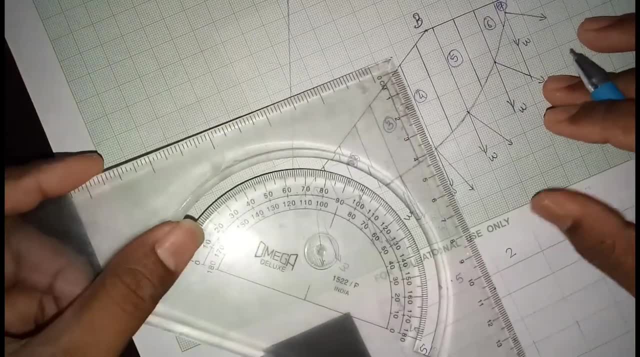 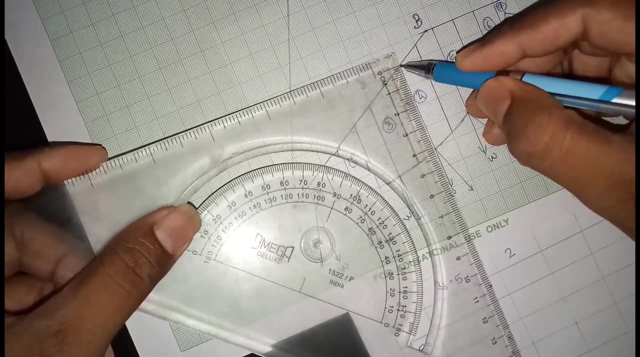 Again, the width is same, two meter. Now consider slice number four. slice number four, having length of mirror ordinate is 4.1. 4.1., 4.1., 4.1., 4.1.. 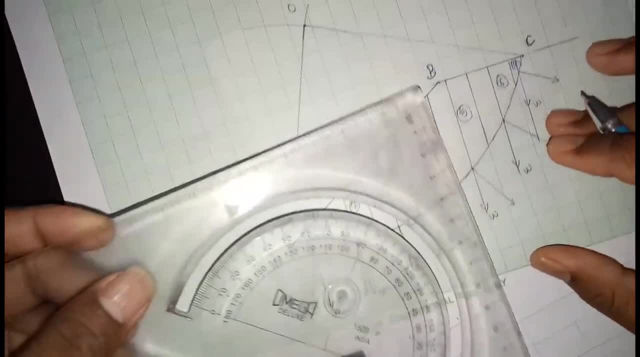 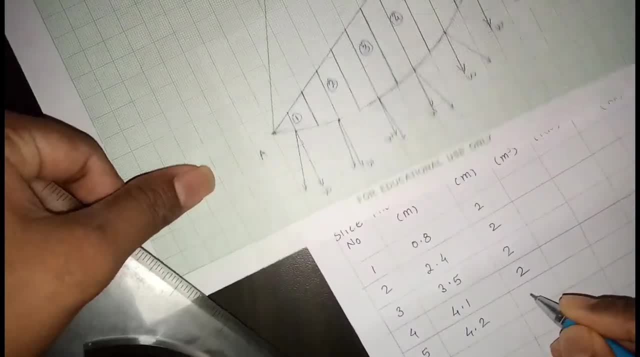 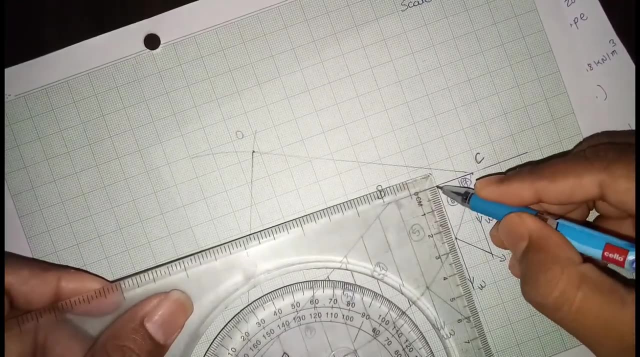 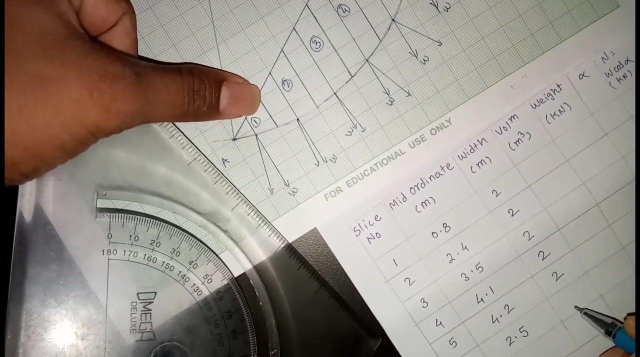 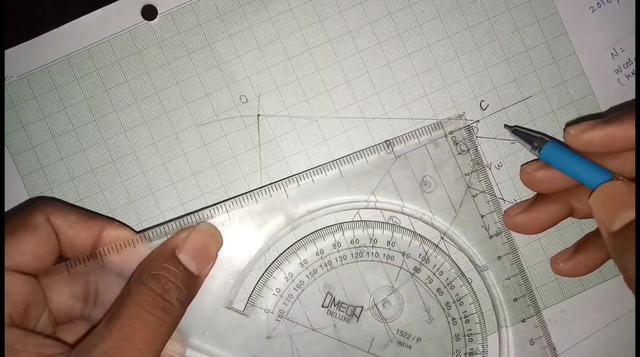 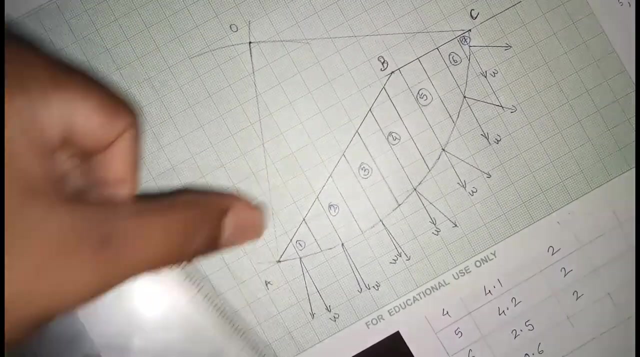 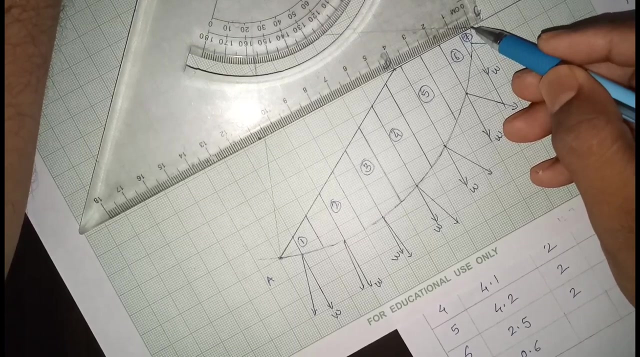 4.2, width is again same two meter. Now slice number six. slice number six having mid ordinate length is 2.5 and length- sorry, width- of the slice is two meter. Now slice number 7, slice number 7 having a mid ordinate length is 0.6 meter, 0.6 meter and width is 0.7.. We know that the width of the slice number, the slice number 7, is 7, 0.7.. 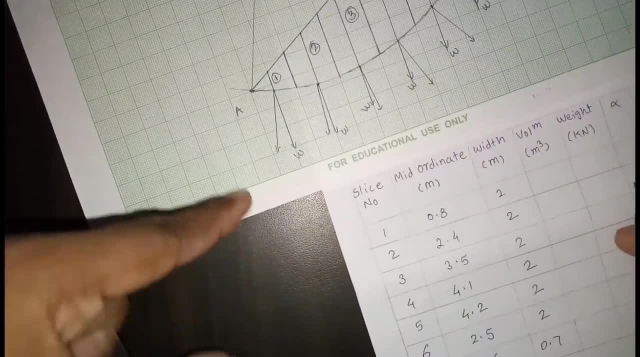 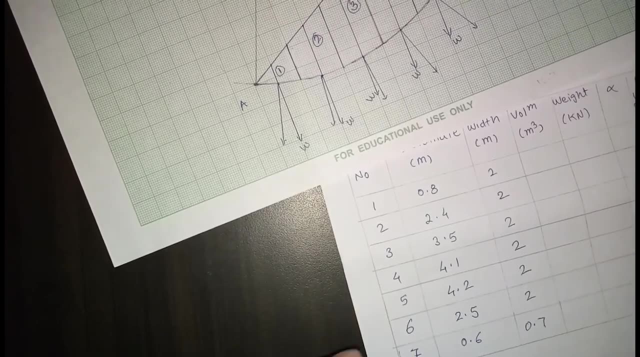 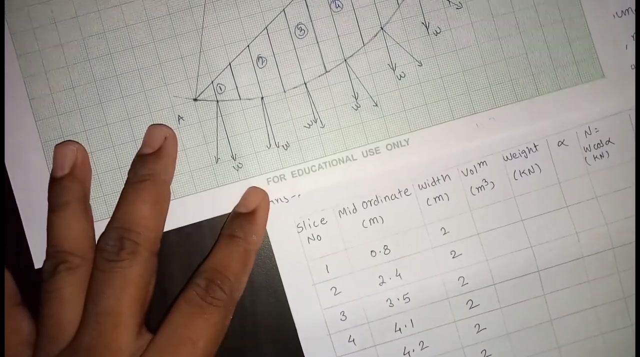 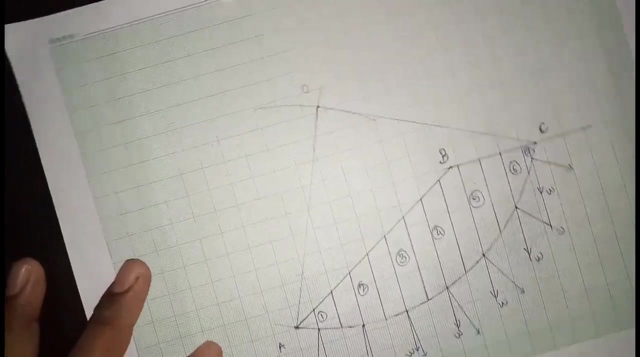 All other slices having standard width. that means equal width, 2,, 2,, 2, 2 meter and remaining slice, slice number 7, having width is 0.7 and mid ordinate height is 0.6 meter. Now we have to measure the angles, alpha angles. How to calculate the alpha angles Now, see here. 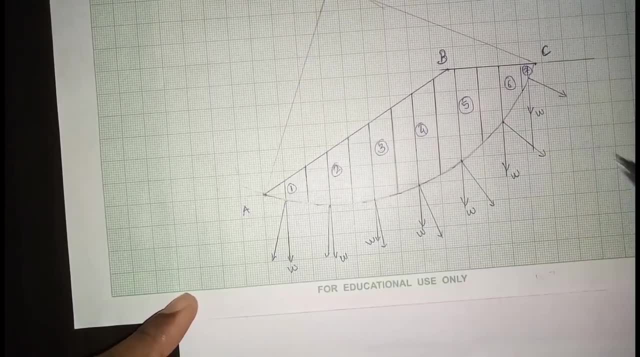 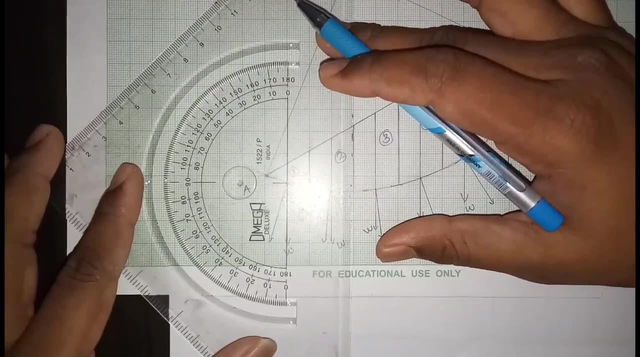 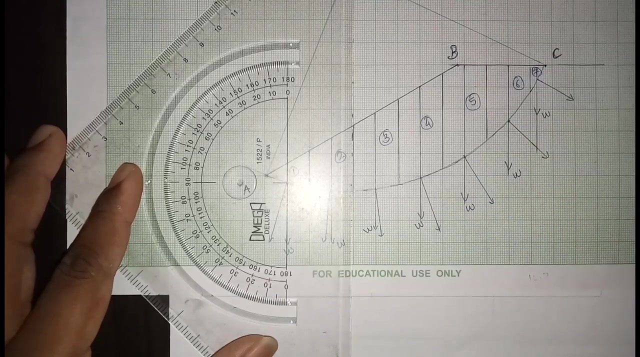 These are the angles for various slices. So we have to measure the angles for various slices. So we have to measure these angles. So, first angle for slice number 1, keep your protector here, center it. Okay, we have to extend the lines so we will get a better idea. 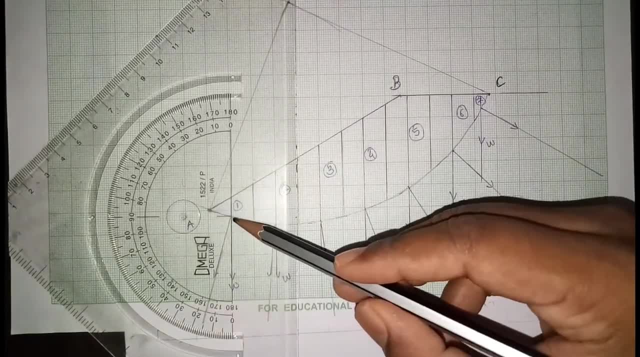 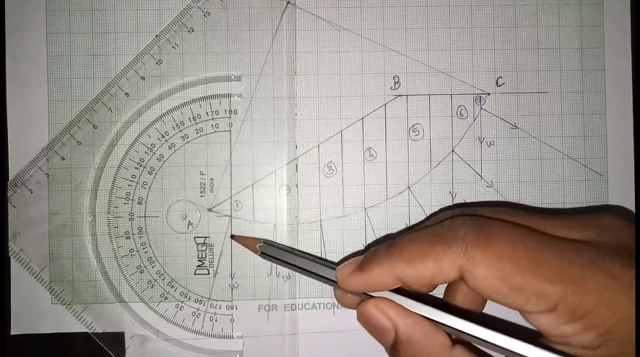 Here we can see that for slice number 1, this is the slice number 1 and this is the inclination angle. we have to measure this angle. So for slice number 1, alpha is equal to 15 degree. Here we can see 15 degree. 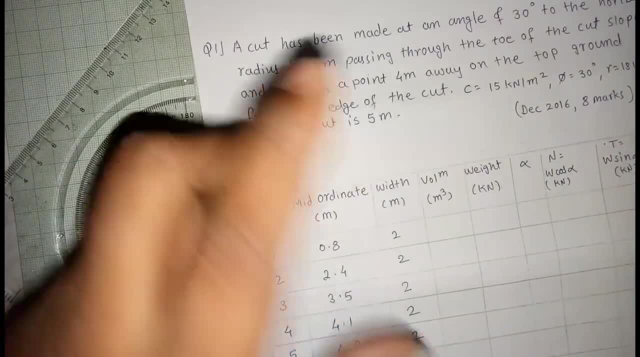 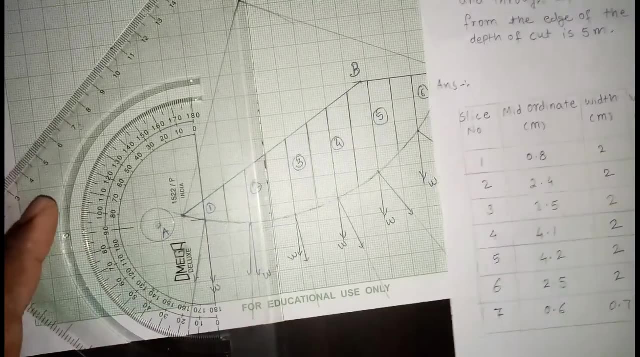 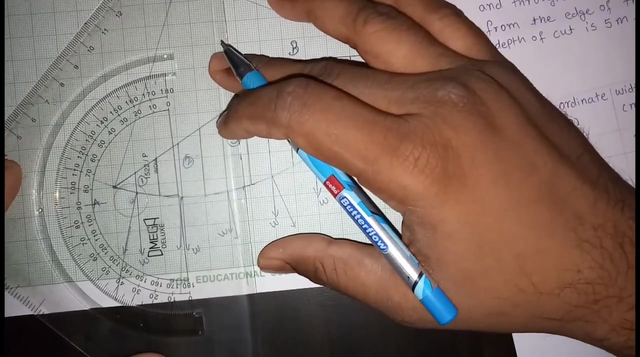 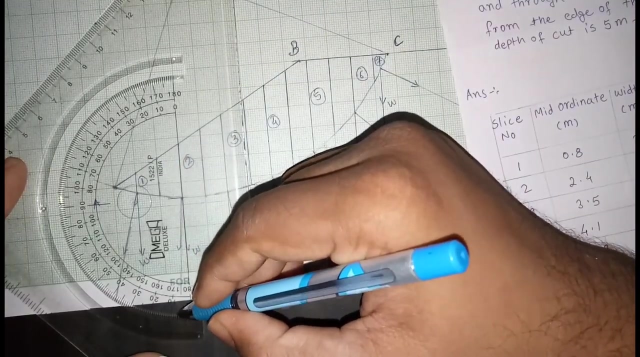 So write down 15 degree In slice number 1, alpha is 15 degree. Now for slice number 2.. So for slice number 2. So for slice number 1, alpha is 15 degree, The angle is 6 degree. 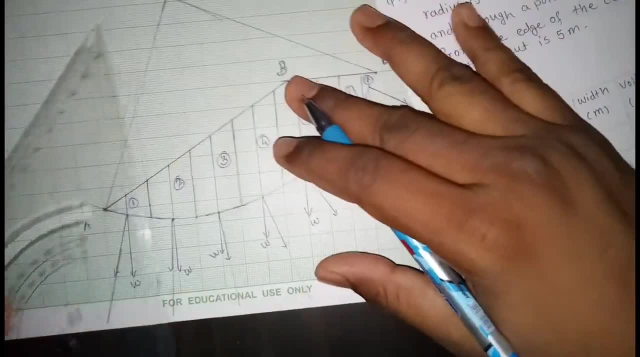 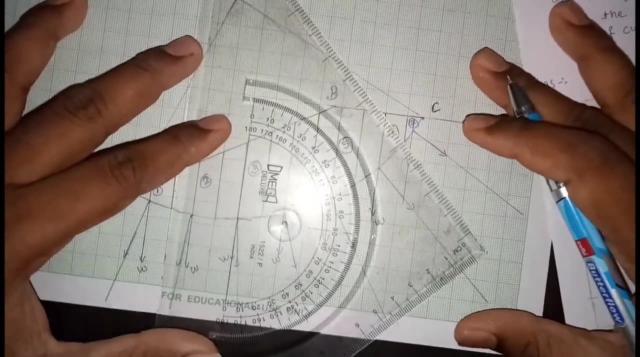 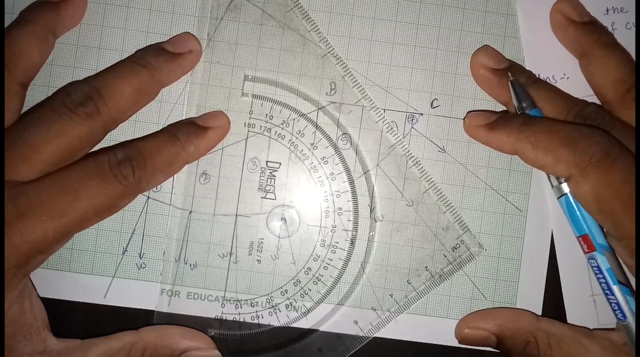 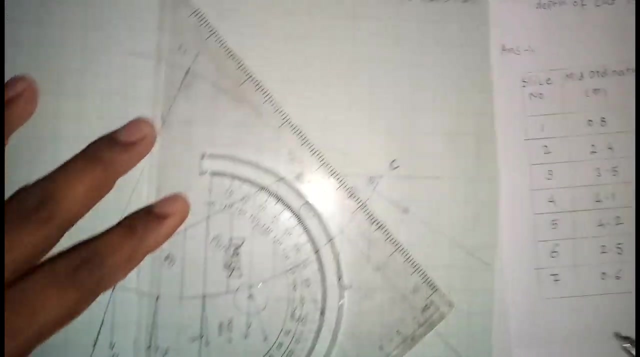 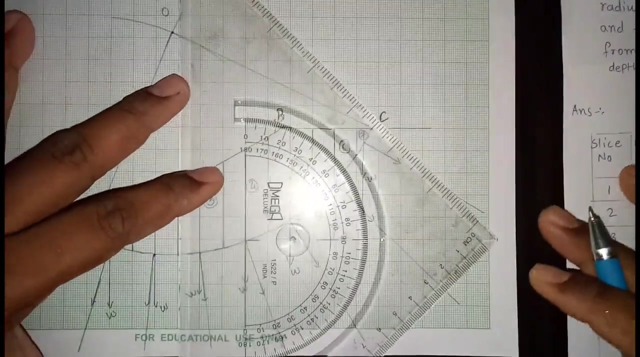 For slice number 2, angle is 6 degree For slice number 3.. For slice number 3.. This is somewhere 9 degree For slice number 3.. For slice number 3.. Alpha is 9 degree Now for slice number 4.. 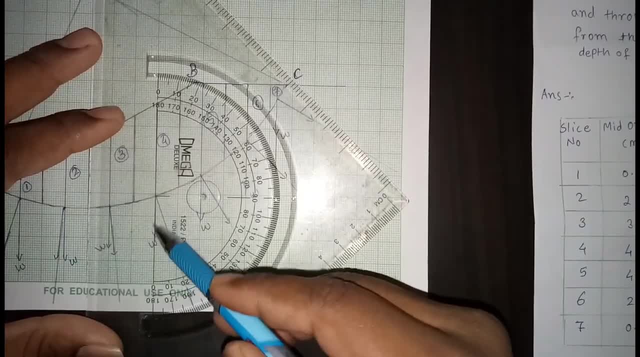 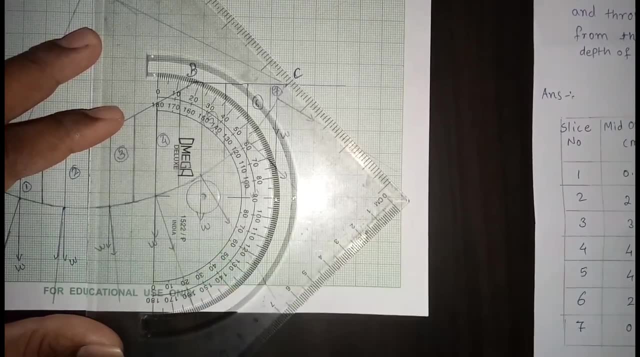 Slice number 4, angle is 20 degree. here This is W going downward and this is alpha. So this angle is 20 degree For slice number 4.. Write down: For slice number 4, angle is 20 degree. 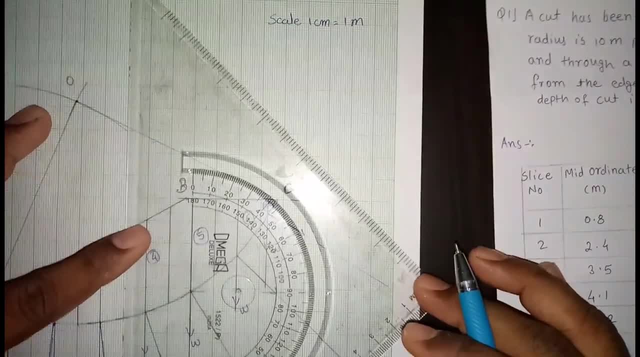 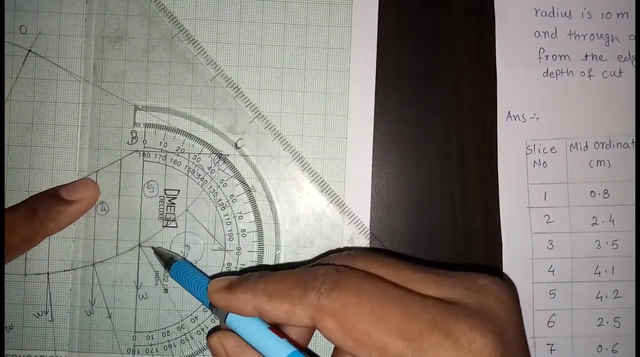 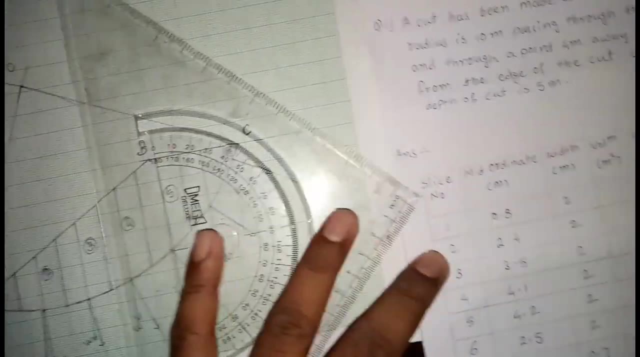 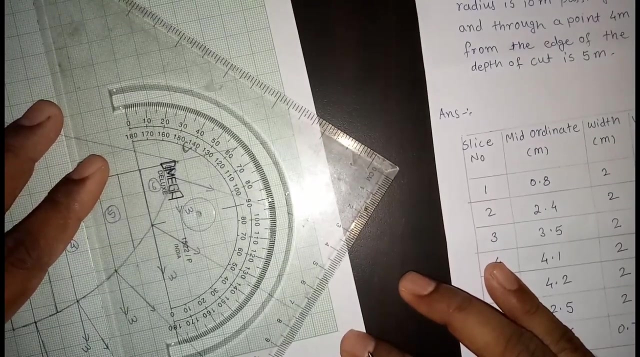 For slice number 5.. This angle is 25 degree. angle is 32 degree. Angle is 32.. This is slice number 5.. W is going downward and this angle is 32 degree. Write down 32 degree. Then for slice number 6.. 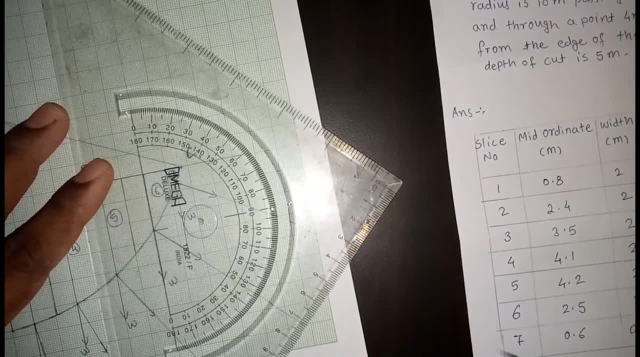 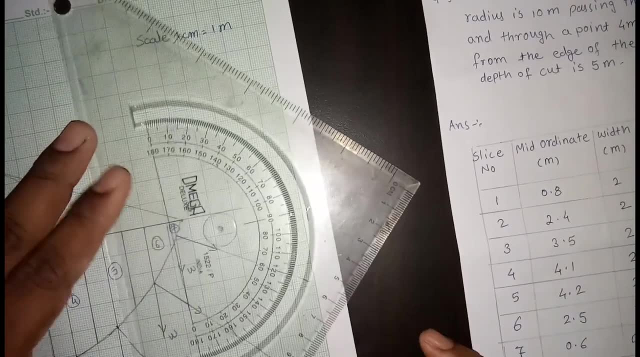 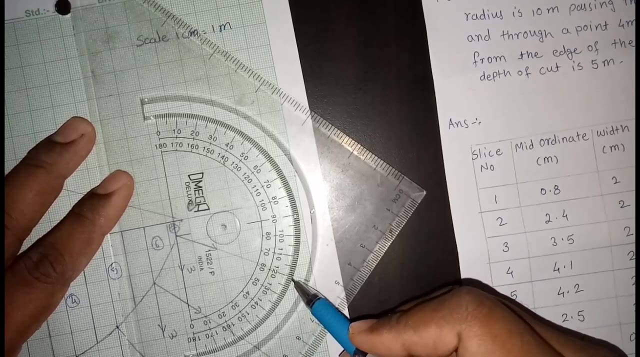 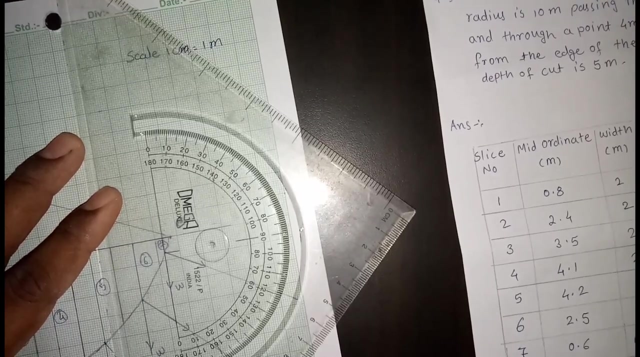 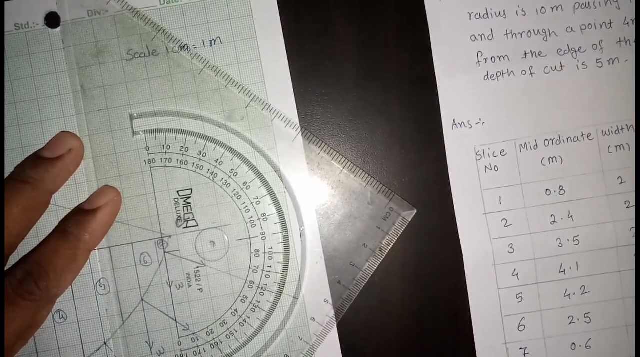 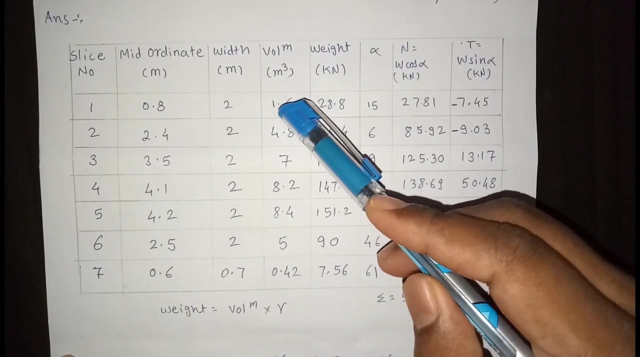 Angle is 46 degree For slice number 6.. six degree and slice number seven, the inclination angle is 61 degree. for slice number seven, inclination angle is 61 degree. after calculations of mid or diners and alpha, calculate the volume. ok, now hold, volume is mid ordinate. 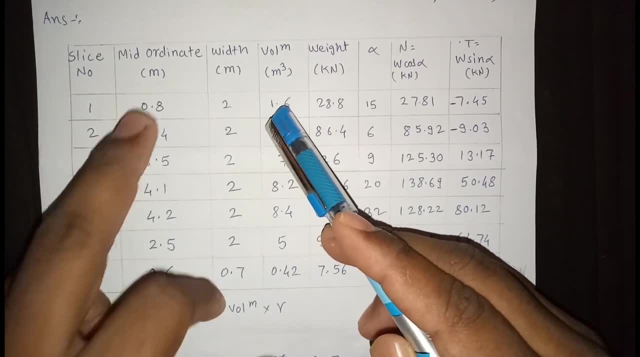 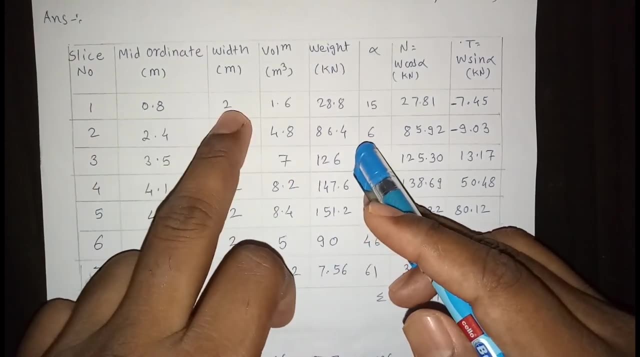 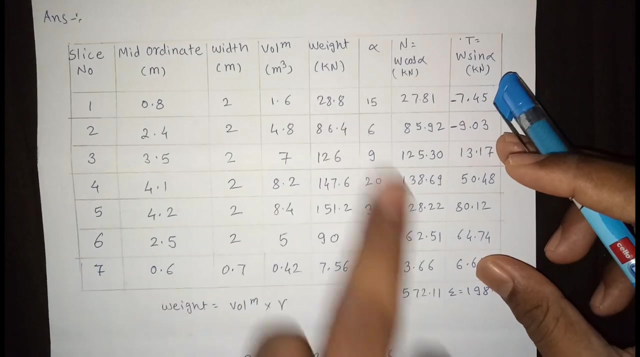 multiplied by virth, you will get volume. okay, this is the area and this is the present height. so mid ordinate multiply by width, you will get volume for all the slices. okay, now how will? how you will get the weight- weight is equal to volume- into unit weight of the soil. so this is: 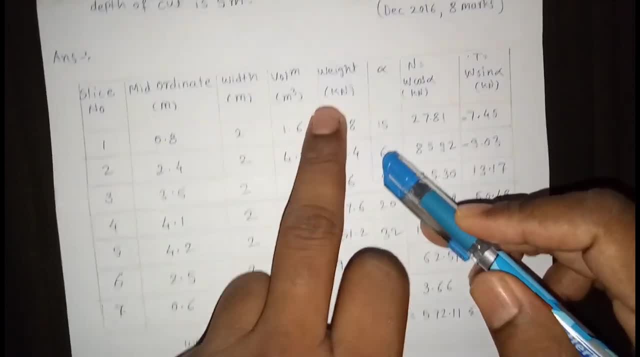 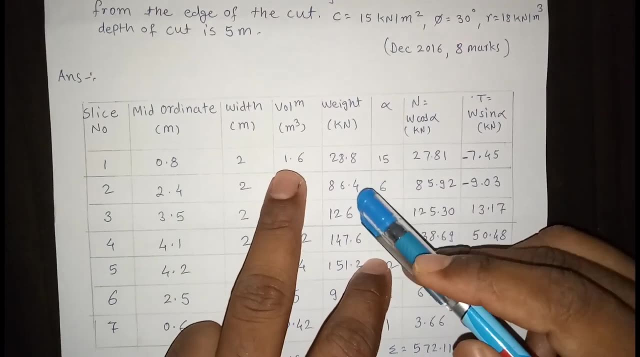 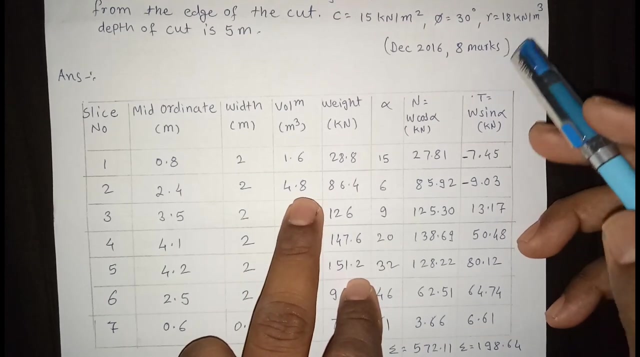 volume. 1.6 into unit weight of soil is 18. it is given to you. unit weight of the soil is 18 kilo Newton per meter cube. so 1.6 into 18 weight is 28.8, 4.8 into 18. 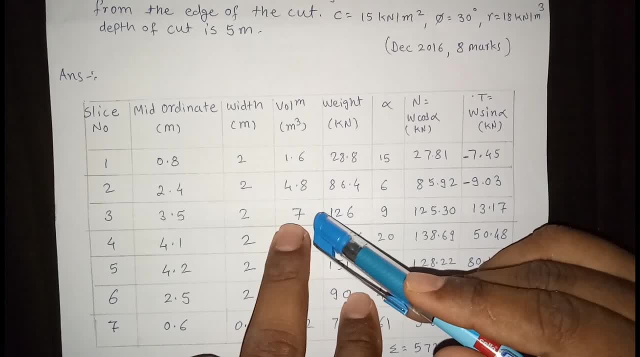 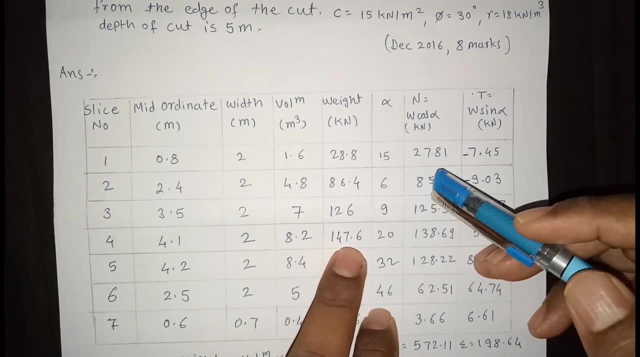 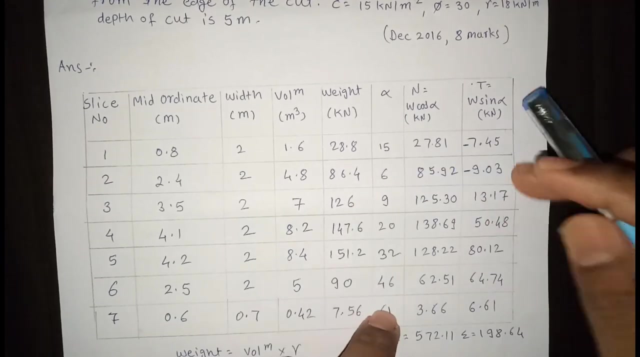 weight is 86.4. 7 multiplied by 18, so you will get 126. 8.2 multiplied by 18, you will get 147. likewise, calculate the weight for all the slices alpha. we know that we have already calculated with. we know that we don't. we have already. 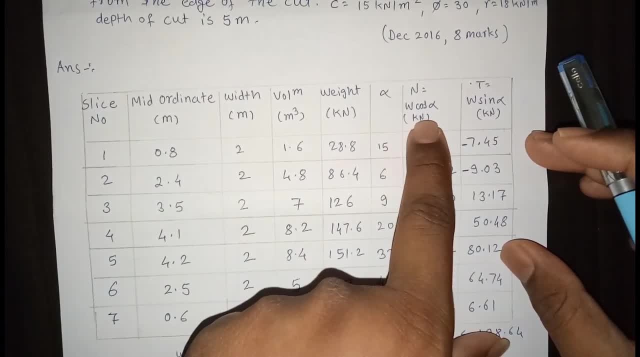 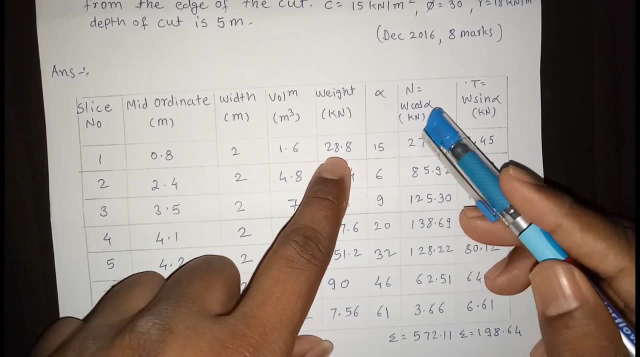 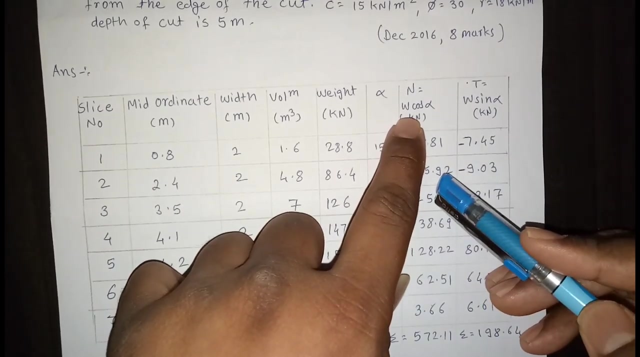 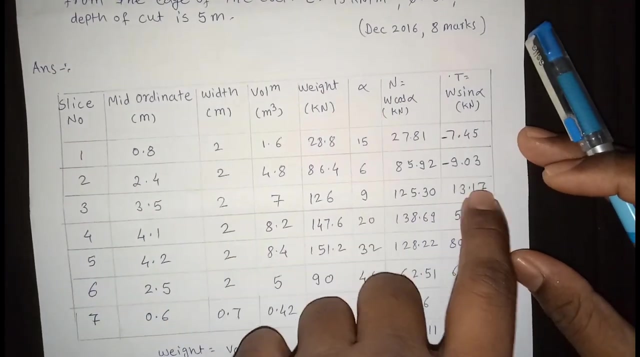 calculated. now calculate normal. normal is equal to W cos alpha W. we know 28.8 cos alpha is 15 degree, so 27.81. now change the weight. as you can see, we have already calculated the weight for all the slices- and change the angle, you will get all normals. and for tangent, t is equal to W. 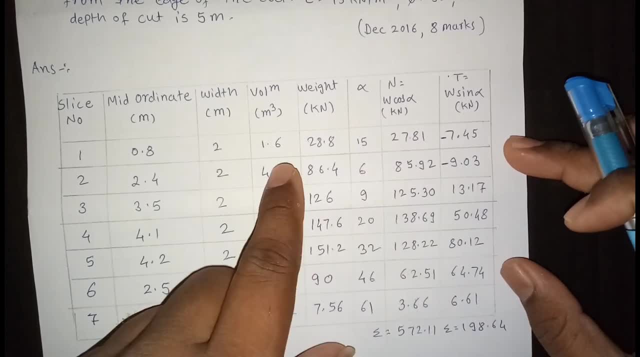 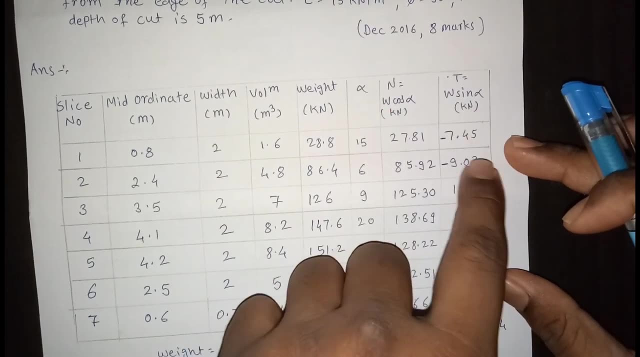 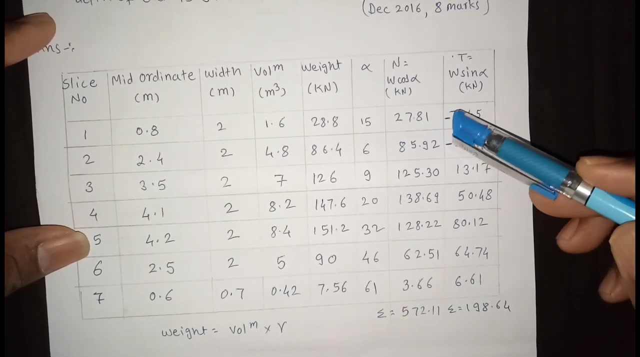 sine alpha- here also same W is 28.8. sine alpha is 15. only instead of cost you have to put here sine, so you will get all the values now. here. the difference is that the for slice number 1 and slice number 2 minus or negative signature. 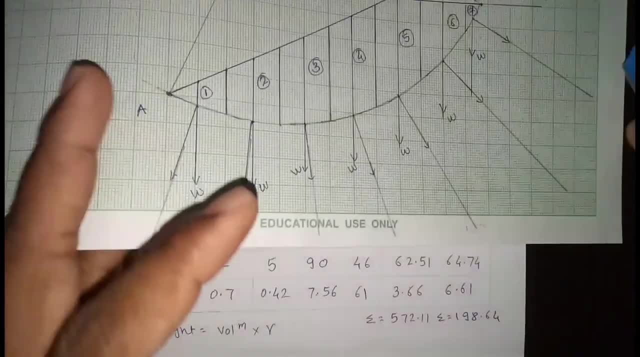 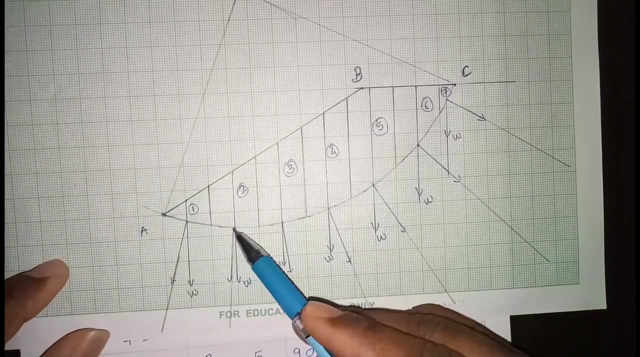 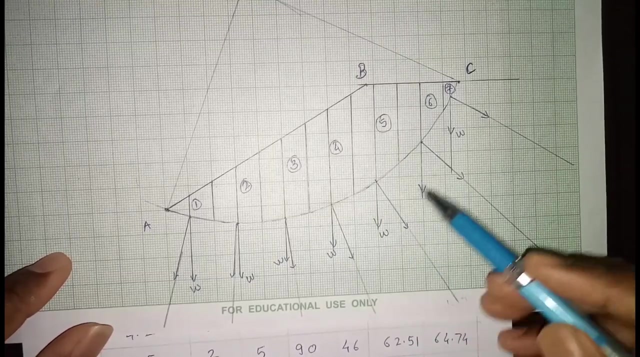 level 2. anything is negative sign. that means only negative sign will be not given to them. because here we can see: given maybe negative shows that you will imagen classes. you will also see that all the angles are excluding slice number one and slice number two. all the angles are towards right side of the way to see. 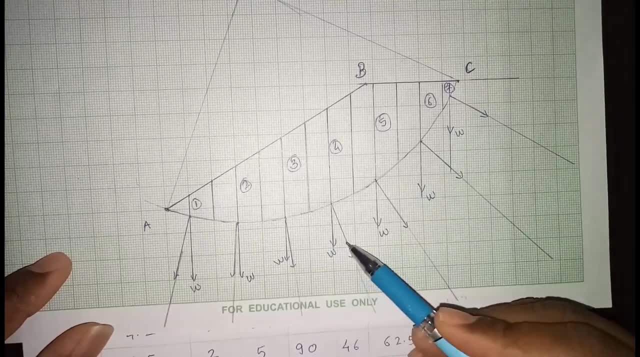 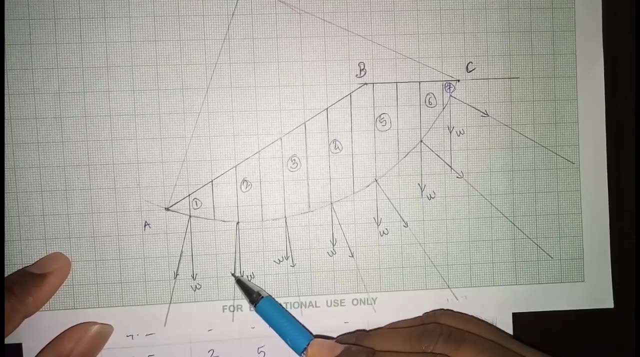 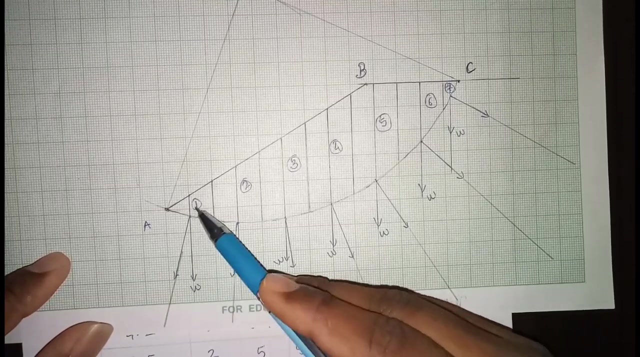 here slice number seven, having angle towards right side of the weight. here also same, here also same, here also same number two: angle is towards left side of the weight. for slice number one also, angle is left side of the weight. so for slice number one and slice number two, negative signature. 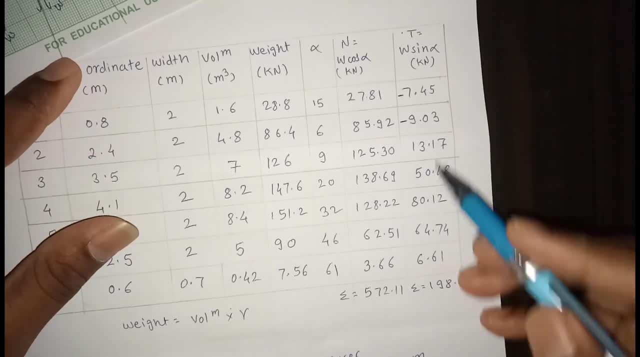 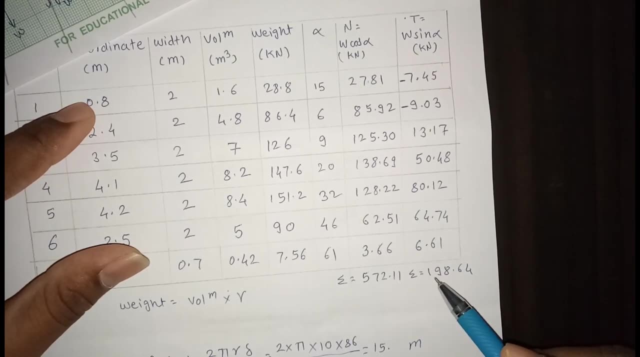 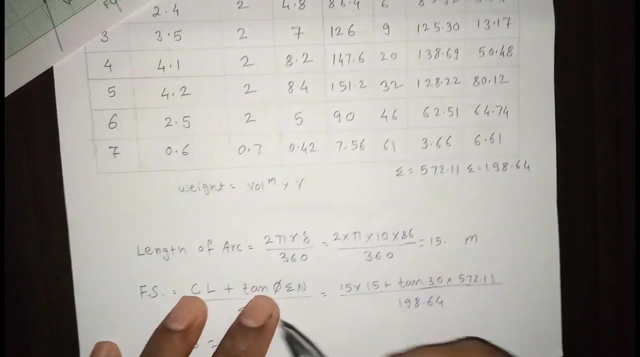 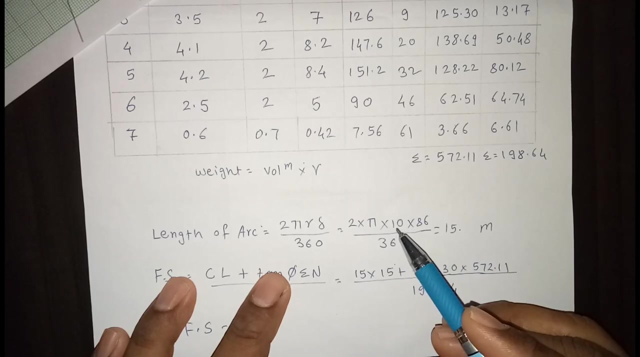 is given okay, so we have to minus this. so, after summation, n is equal to 572.11 and summation of t is equal to 198.64. after, after summation, calculate length of arc. length of arc is equal to 2 pi r. delta by 360, 2 pi r is 10 and delta is 86. delta is the angle between these two. 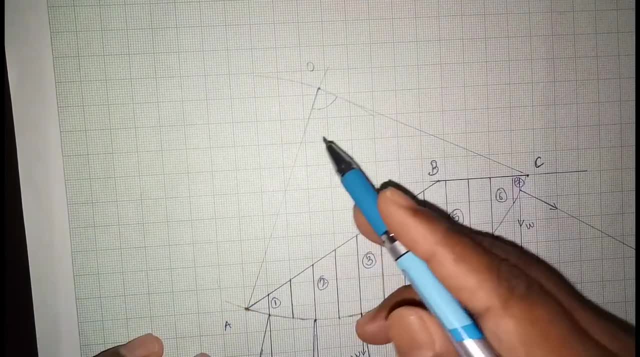 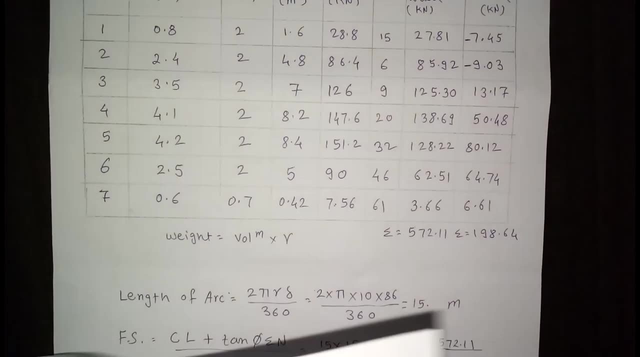 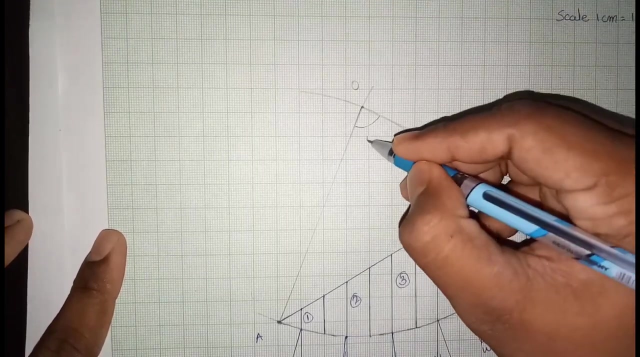 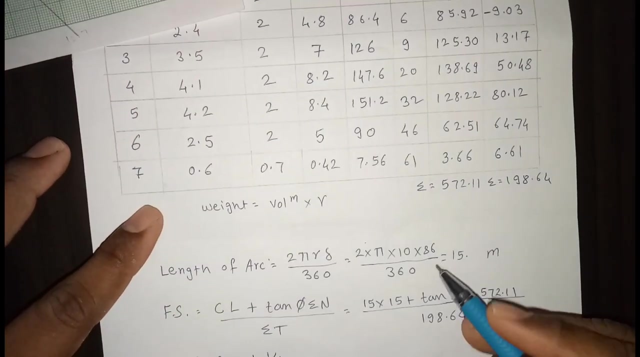 points or angle between these two lines o a and o c. okay, so this angle is 86 degree. the line o a and o c having angle is 86 degree. this is called deflection angle or delta. so this is: delta is 86 divided by 360. the length of the arc is 15 meter. okay, 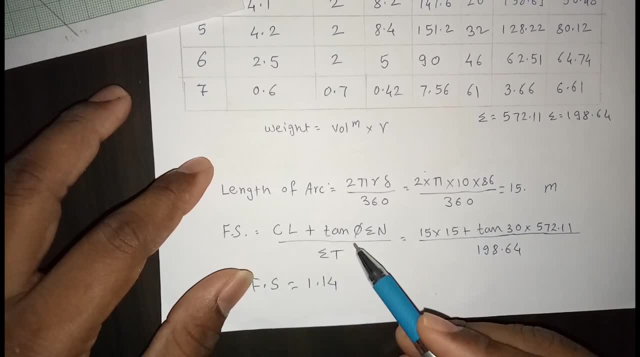 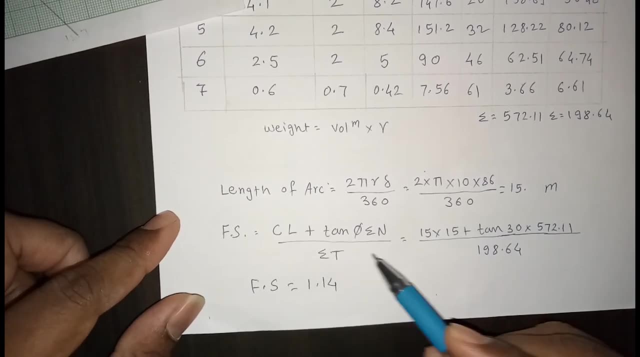 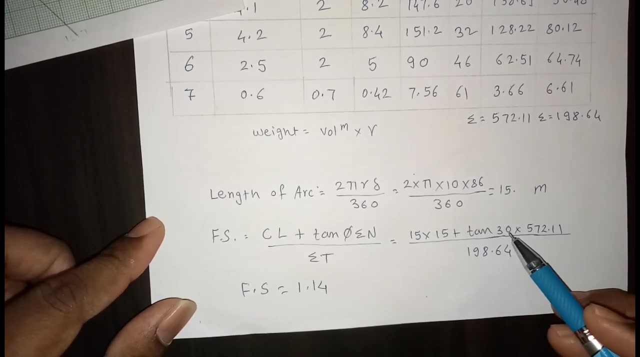 so factor of safety is equal to cl plus tan phi. summation of n, summation of n divided by summation of t. okay, so this is the angle between these two points. so after summation of t. so c is the cohesion. cohesion is 15, into length of arc is 15 plus tan phi is 30. 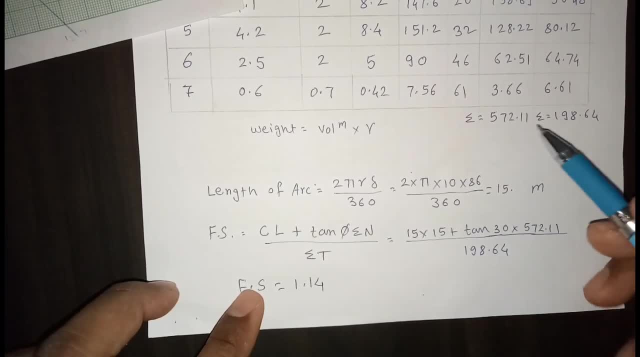 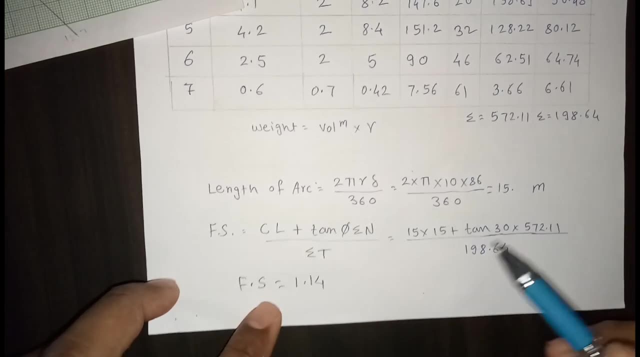 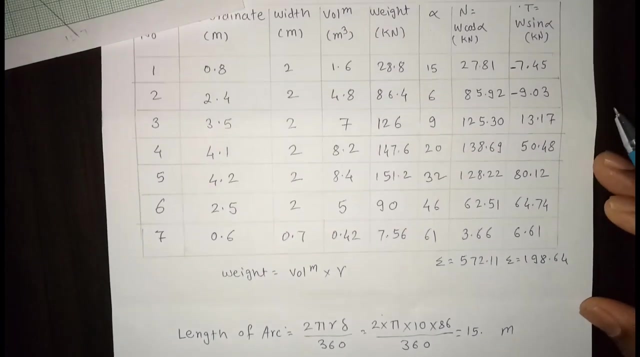 degree into summation of n. summation of n is 572.11. divided by summation of t is 198.64. at the end, factor of safety by swedish circle method is 1.14. thank you, thank you very much.